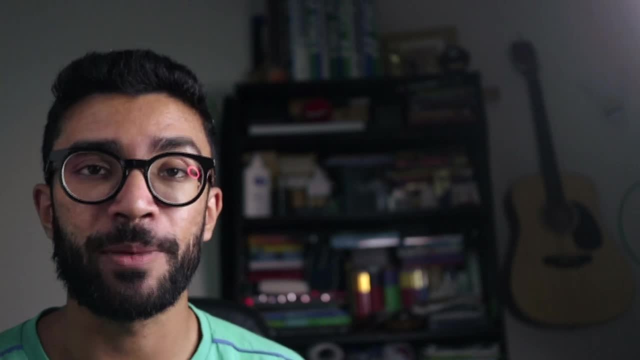 physical phenomena. But before we begin, I have to tell you that I try and explain this phenomena so literally anyone can understand them. I don't care if you study physics to undergraduate level or if you stopped learning it after high school, And I genuinely think that if I've done a good 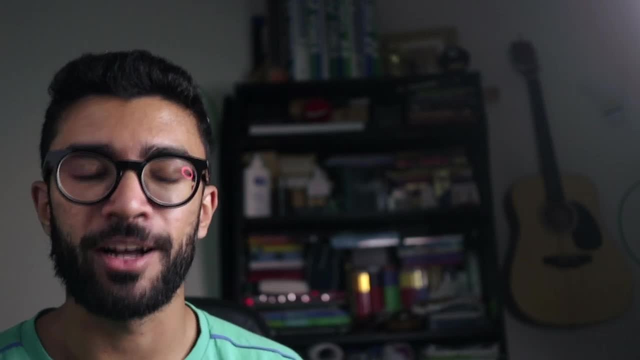 enough job of trying to explain this concept, then you can understand it. However, these are extremely advanced. concepts Like this is stuff that I learned in my third and fourth years of university. So my final year of my undergraduate degree and my one year of my 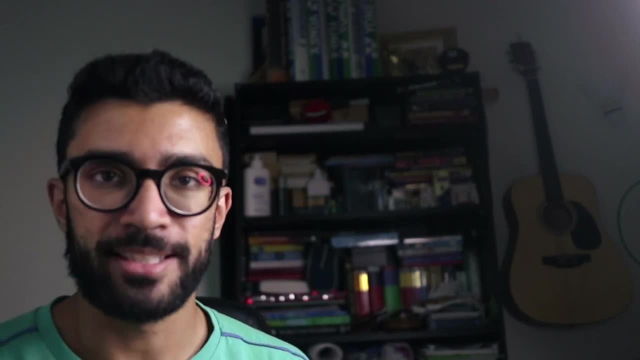 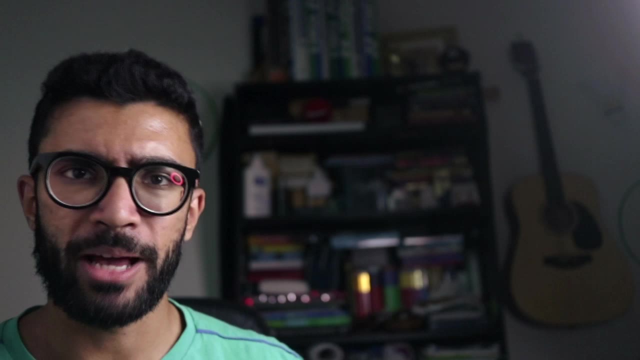 master's degree And for this reason it might take a little while for the concepts to fully settle in and, additionally, you won't get the full gist of it, mathematically speaking. I'm not going to be discussing the detailed maths behind this, But the interesting thing is the stuff that 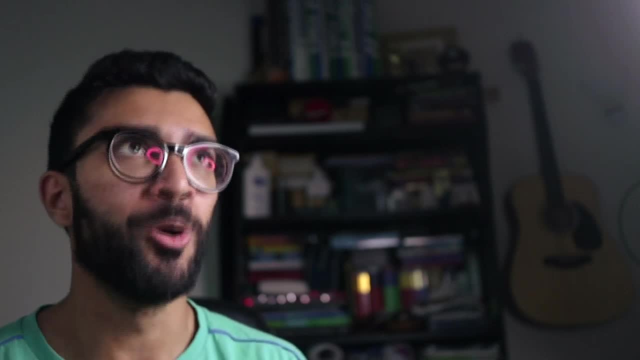 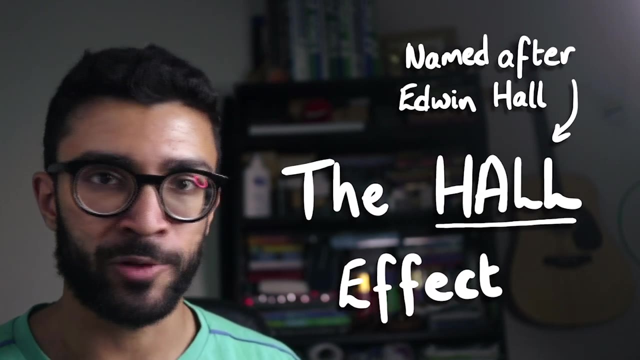 happens on a physical level, and that's what I'm going to be talking about. So now let's finally get into this. The first phenomenon that we're going to be looking at is known as the Hall Effect. Now it's named after a dude called Hall. 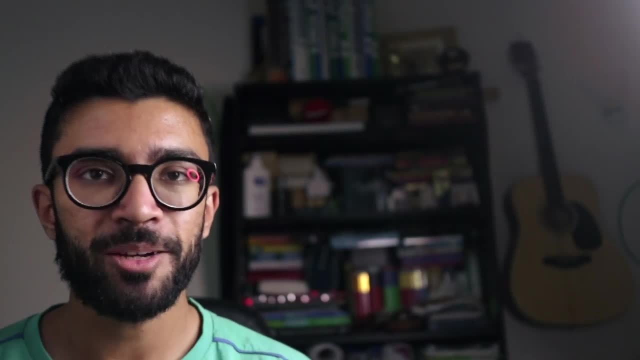 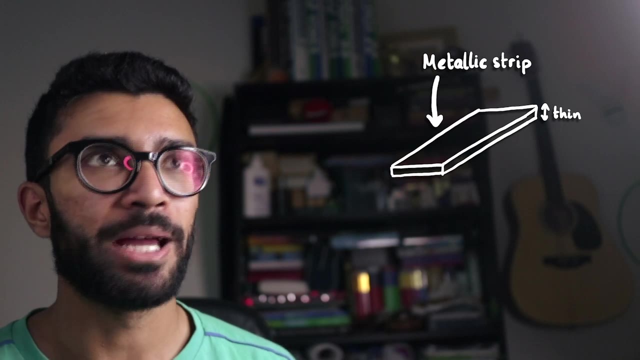 it's got nothing to do with corridors and landings or anything like that. Let's start by imagining a very thin strip of metal shaped like this, And let's also remember that metal, just like other forms of matter, are made up of atoms. However, specifically in metals, the electrons in the outer 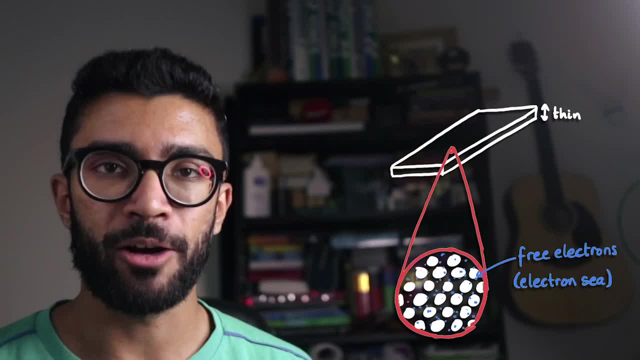 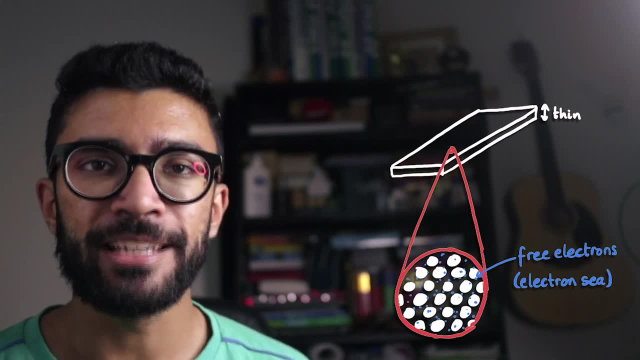 shells of these atoms that form the metal are actually free to move around. They form what's known as the electron sea, because electrons are flowing and moving around all the way around the metal, And so what this essentially means is that electrons being charged particles can actually 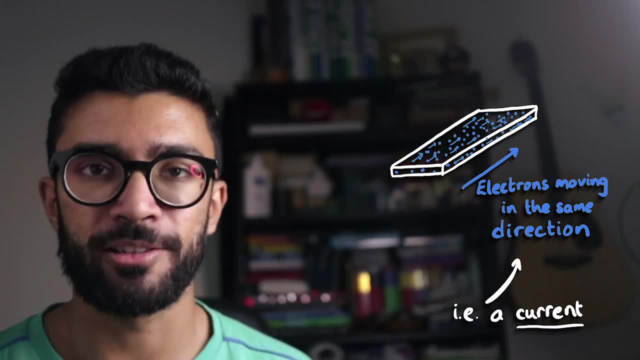 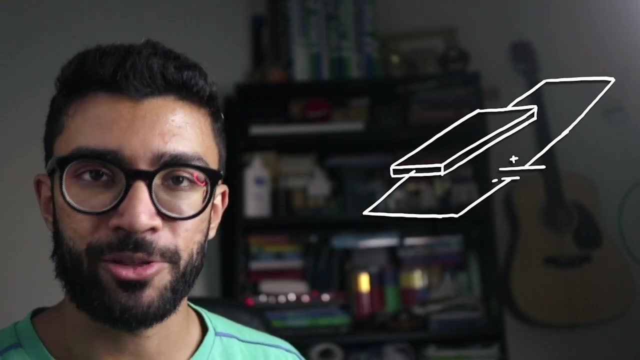 flow in one direction through the metal and carry a current. That's what a current is: it's a flow of charged particles. So now that we've established that, let's imagine that we connect a battery or a cell to our strip of metal in this way And the battery or cell connected in this particular 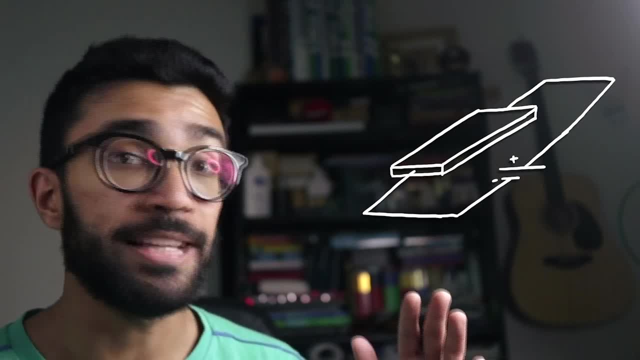 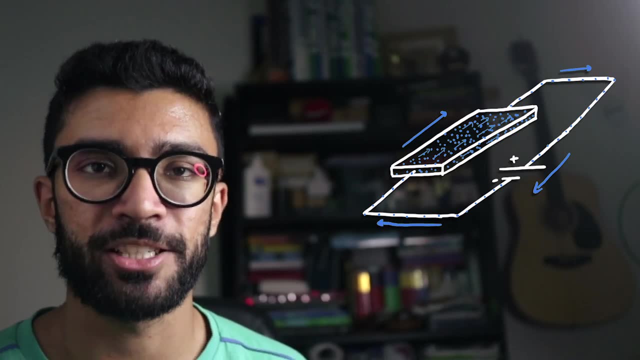 orientation causes electrons to flow in that strip of metal in this direction, And so we have what we said earlier would be a current. We have a flow of charged particles, in this case electrons, in one direction through the metal. So far, so good. right, We've just used our strip of metal as a 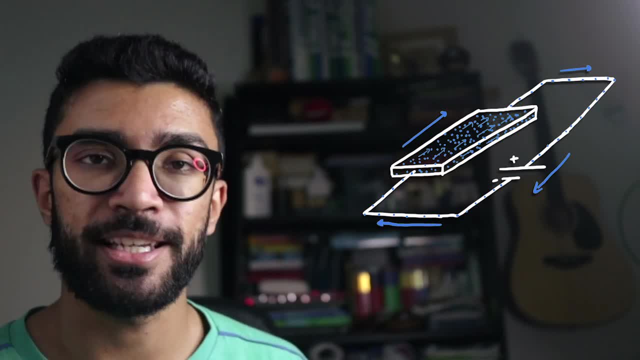 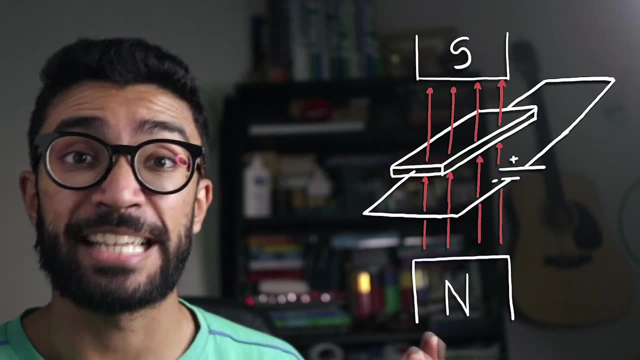 circuit. But now what happens if we take our entire circuit and place it inside a magnetic field pointing in this direction? In other words, the north pole is here and the south pole is here. If you want to know a little bit more about magnetic fields, by the way, check out my videos. 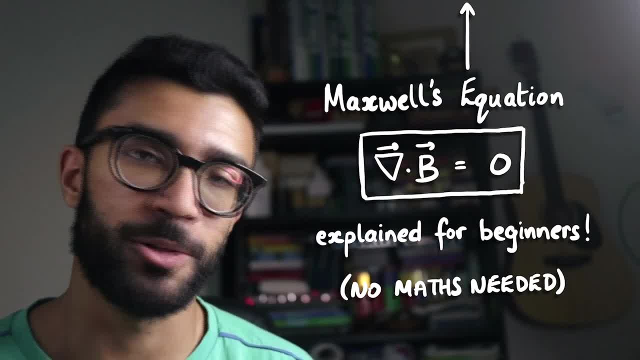 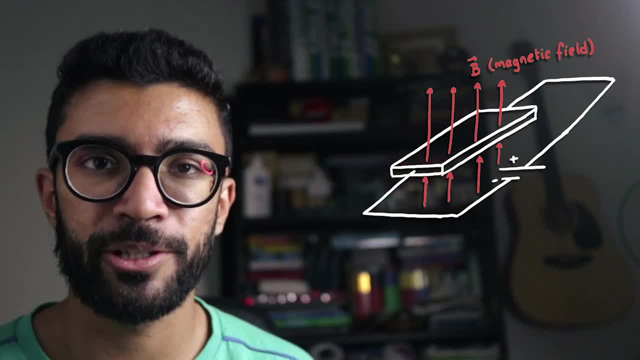 on Maxwell's equations. They deal with everything- electricity and magnetism- so check those out if you haven't seen them already. But anyway, so we've taken our metallic strip and placed it in a magnetic field. We said earlier we placed the whole circuit in the field. but to simplify things, 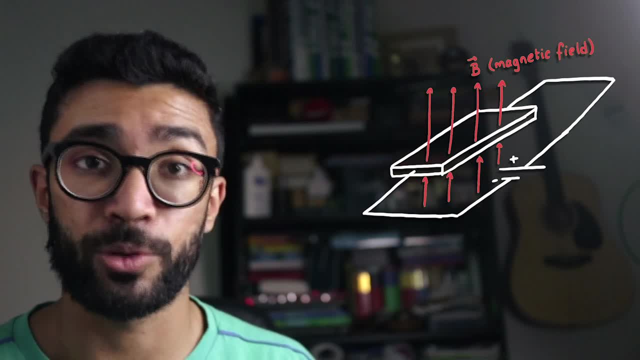 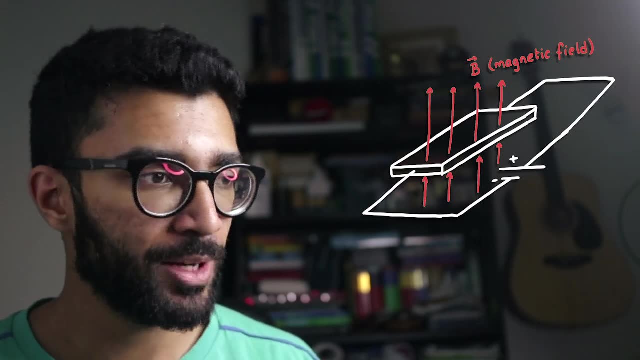 let's just imagine that the magnetic field only exists so that it passes through the metallic strip. Now what a magnetic field does to an already moving charge is to exert a force on it. So let's imagine that we look at one of the electrons moving through our 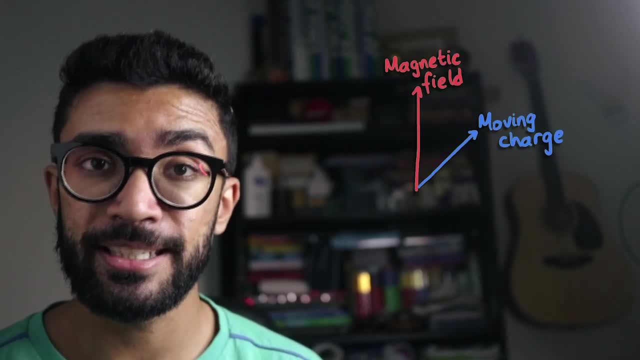 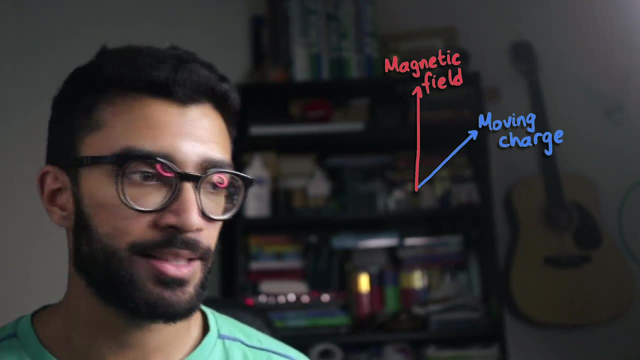 metallic strip. Now, this electron, as we already know, is the charged particle and it's moving because it's part of the current flow. It's part of a group of charged particles flowing in a certain direction, which means that we have all we need in order for the magnetic field to exert. 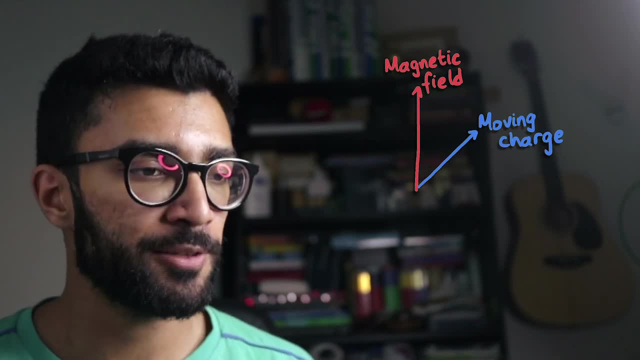 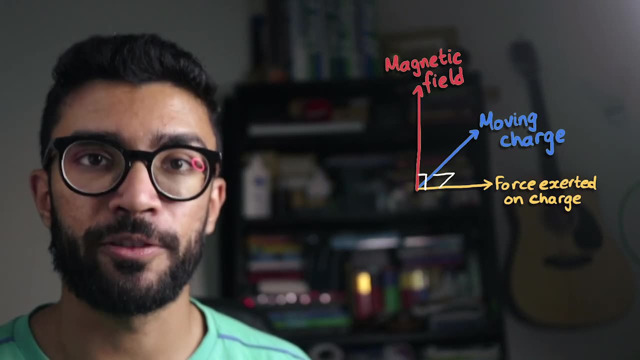 a force on it And, specifically speaking, a magnetic field exerts a force on a moving charge that's perpendicular to, or at right angles to, both the direction of the flow of charge and the magnetic field. And so if electrons are flowing in a particular direction, we've got the magnetic. 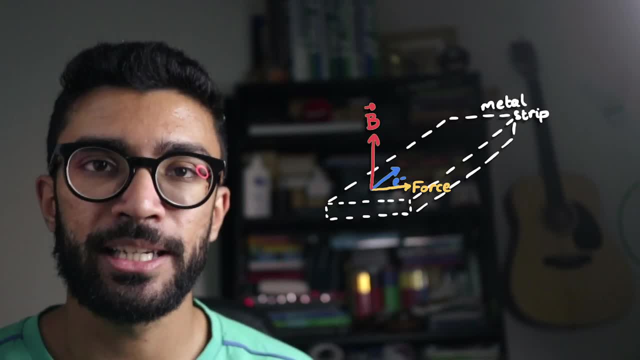 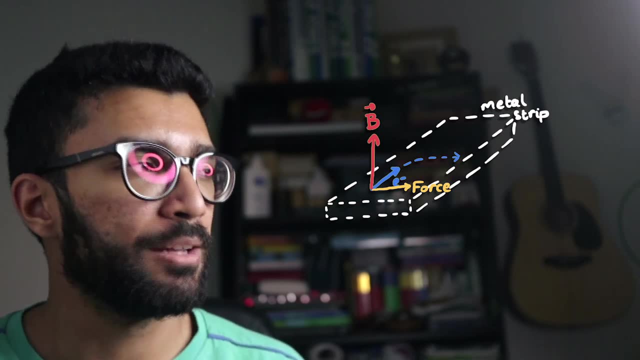 field perpendicular to that, then the force exerted is going to cause the electrons to move in this direction. So, basically, what we had earlier was a straight flow of electrons from one side to the other, and we're talking about a flow along the length of the strip. And now 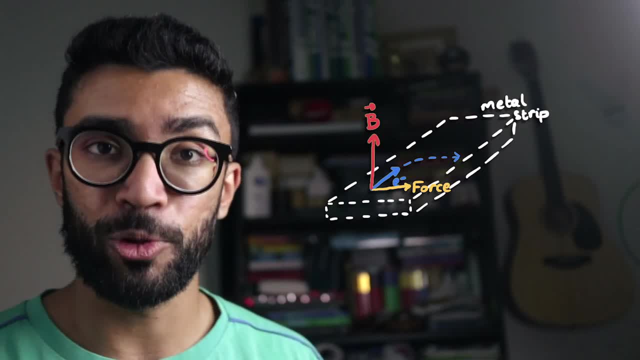 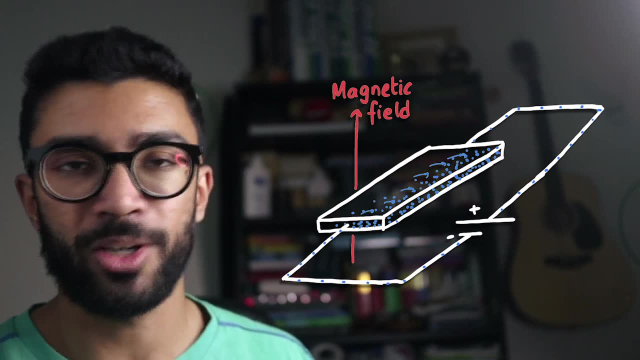 because of the magnetic field, the electrons are going to be moving, not in that direction anymore, but they're going to be curving towards one of the sides of the strip And essentially the magnetic field pulls all of these electrons, or quite a lot of these electrons, toward one end of the strip. 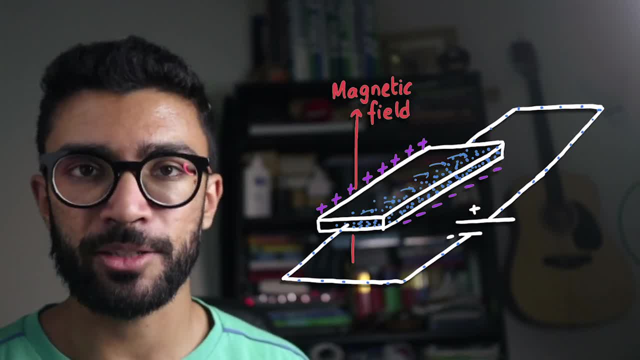 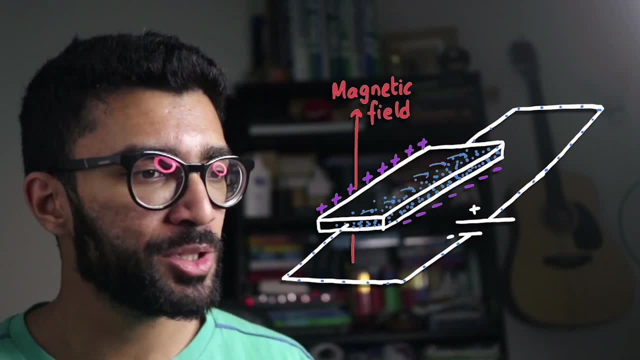 leaving that end negatively charged because electrons are negatively charged particles, and the other end of the strip, because of a deficit of electrons, is going to be left positively charged. Well, this kind of distribution of charge along the width of the strip actually. 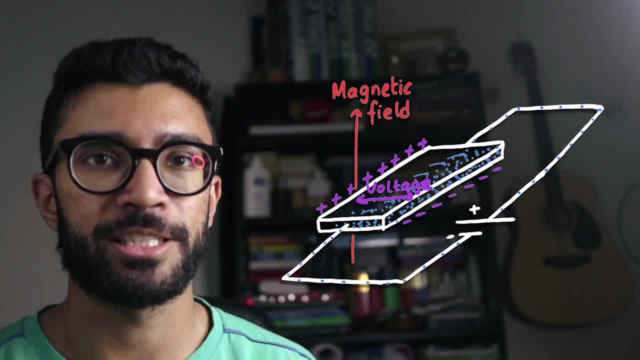 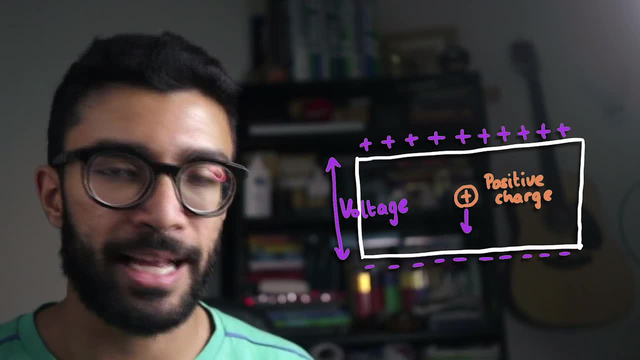 generates a voltage across the width of the strip. Think about it All a voltage is is a measure of how a charged particle placed at a particular point would move based on electric forces acting on it. And a simpler way to think about this voltage generated. 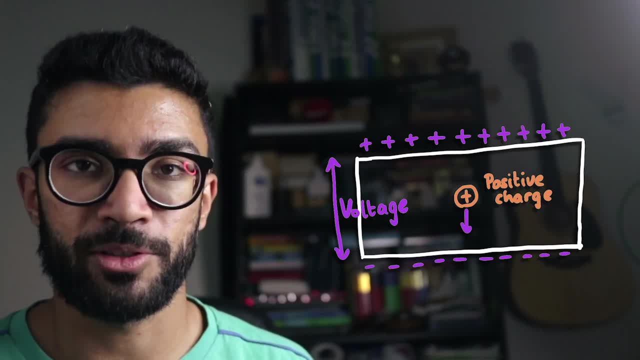 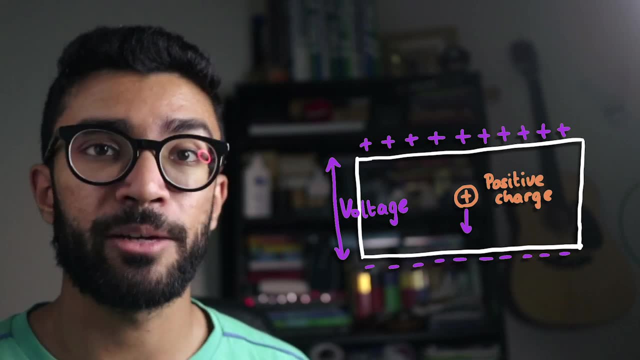 across the width of the strip is that there are lots of negatively charged particles on one end and lots of positive charges on the other end, And so if we were to place, let's say, a random positive charge in the middle of the strip, then it would move away from the positive end and 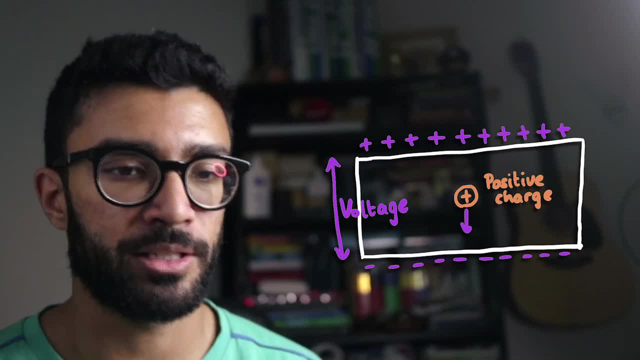 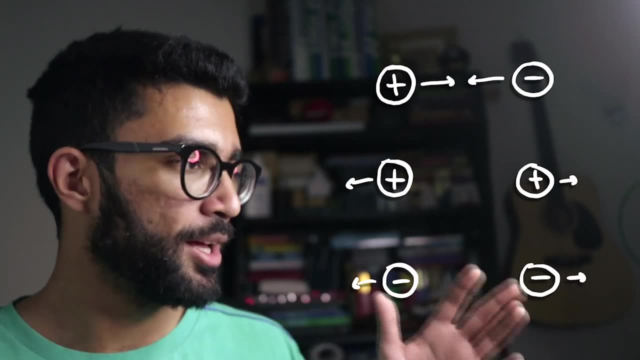 towards the negative end. That's what a voltage is. It causes a charged particle to move due to electrostatic attraction and repulsion. Remember, by the way, that opposite charges attract and like charges repel. So positive charges repel positive charges and negative charges repel positive charges. 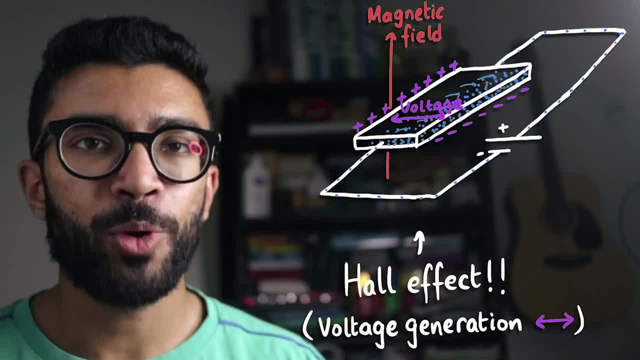 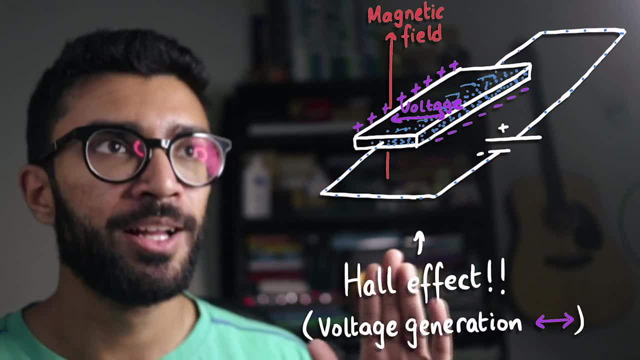 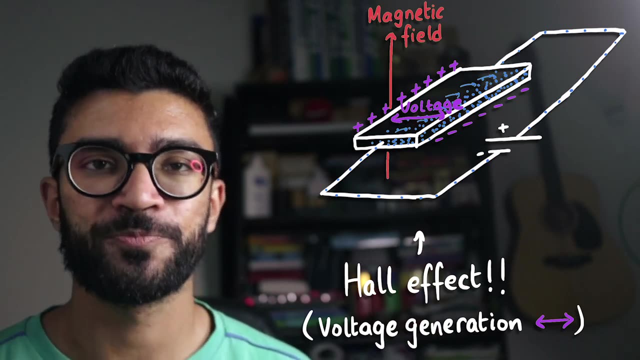 And so what we've discussed so far is basically the Hall effect. It's this generation of a voltage across the width of our strip of metal when placing a strip of metal that already carries a current in a magnetic field perpendicular to the direction of that current, Basically due to the 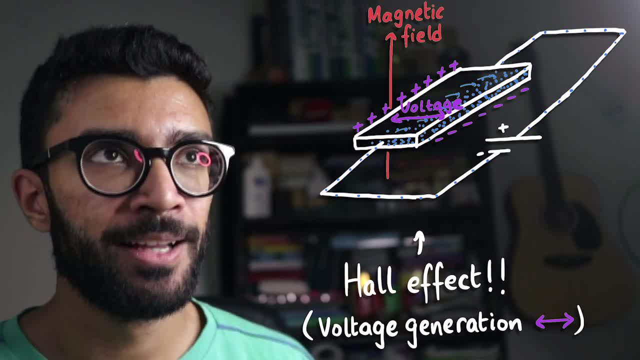 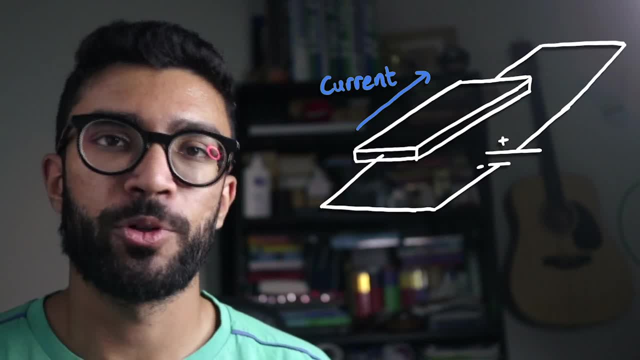 force exerted by the magnetic field on the charges. in the current flow, the charges move towards one end and therefore generate a voltage across the width of our strip. That's the Hall effect. By the way, just for notation's sake, we say that if current was originally flowing in this direction, then the direction in which the 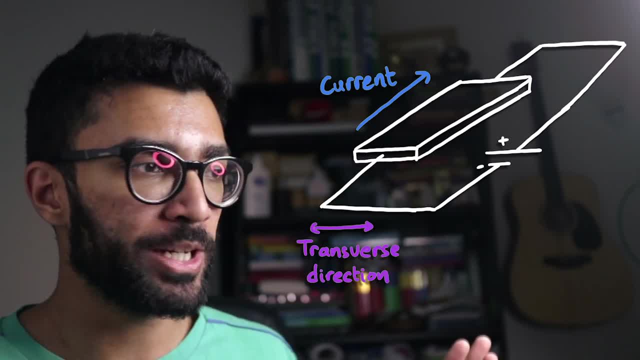 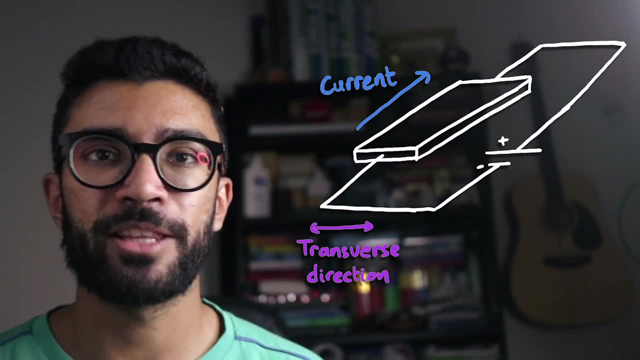 voltage is formed is the transverse direction, And therefore we can measure the transverse voltage generated for any particular strength of magnetic field that we use. Also, if we recall something that's known as Ohms' law, we can recall that this tells us that the 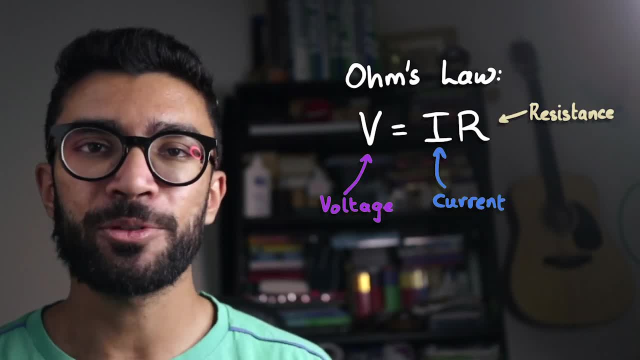 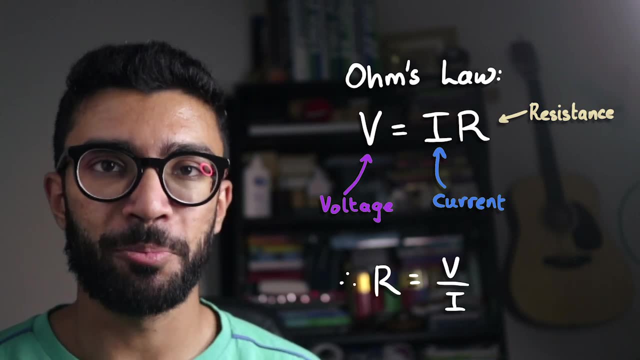 voltage, let's say, across a component in a circuit is equal to the current flowing through that component multiplied by the resistance of that component. And we can rearrange this so that the resistance of that particular component is equal to the voltage across that component divided by the current through it. And in this, 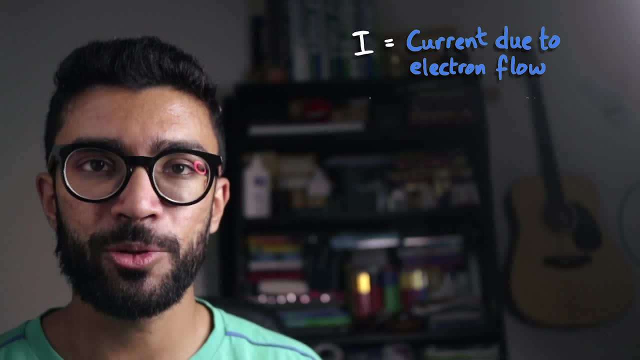 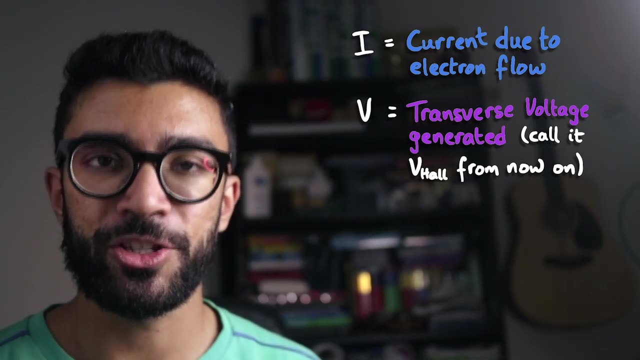 case, we're going to be using some very special values. The current value that we're going to be using was the current initially, when it was traveling straight across the strip, and the voltage value is going to be the transverse voltage that we've measured, because that then, 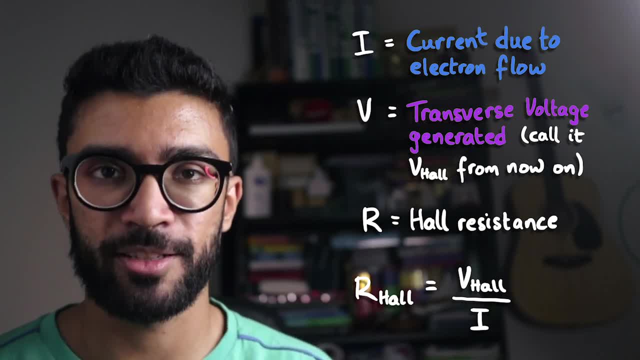 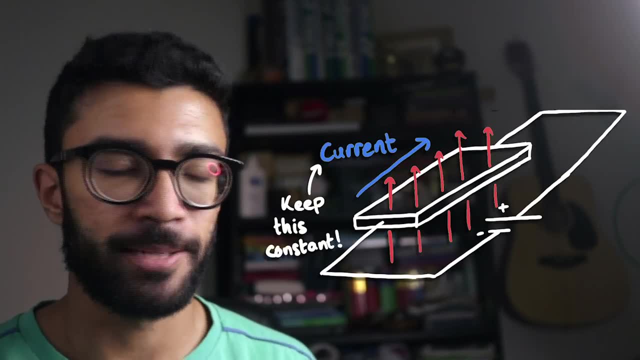 will give us a resistance value known as the Hall resistance, because it's the Hall effect, Anyway. so let's now imagine that we keep our initial current exactly the same. We do not change anything about it. It's the same value all the way throughout an experiment that we're. 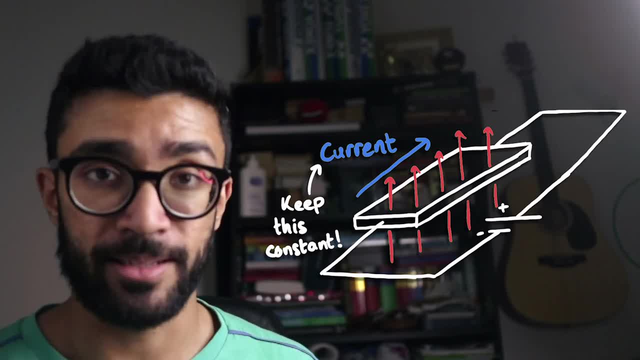 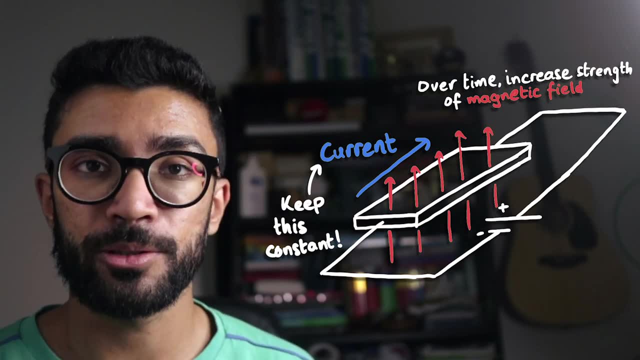 just about to conduct. We also keep the strip of metal exactly the same. We do nothing to it whatsoever. What we do change is the strength of the magnetic field. We start with a very weak magnetic field and then we increase its strength so that it gets stronger and stronger, And as we 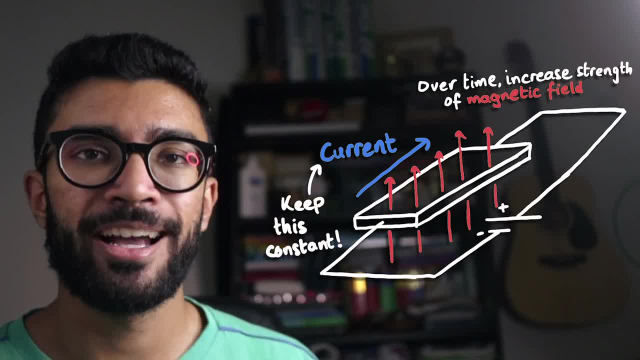 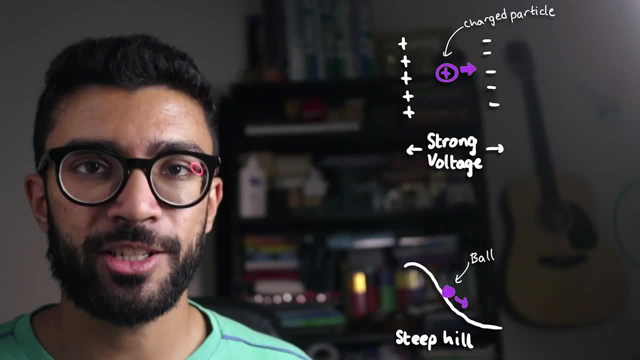 increase the strength of the magnetic field. what we can do is to measure how the Hall conductance changes with the strength of the magnetic field- And remember that a voltage is just a measure of how a charged particle is going to change. So we can measure the strength of the magnetic field. 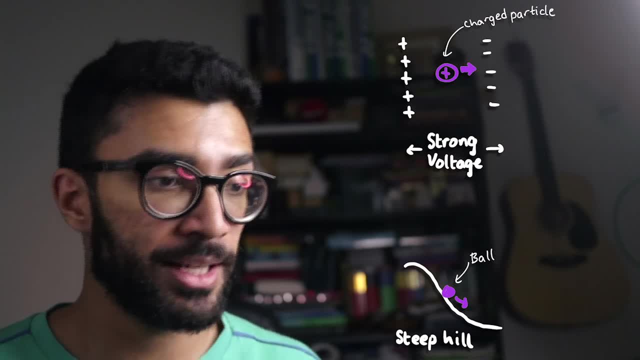 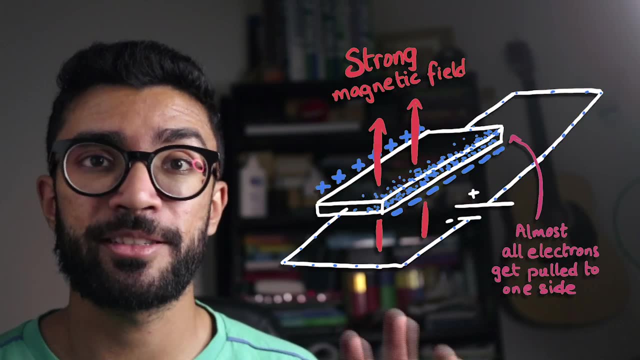 placed in that particular region wants to move. The larger the voltage, the more it will accelerate. It's kind of like a ball rolling down a steeper hill. You get the idea, But anyway. so what we would expect is, as we increase the strength of the magnetic field, the force exerted by the magnetic 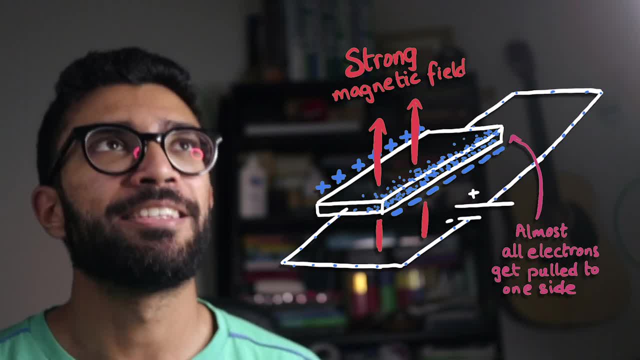 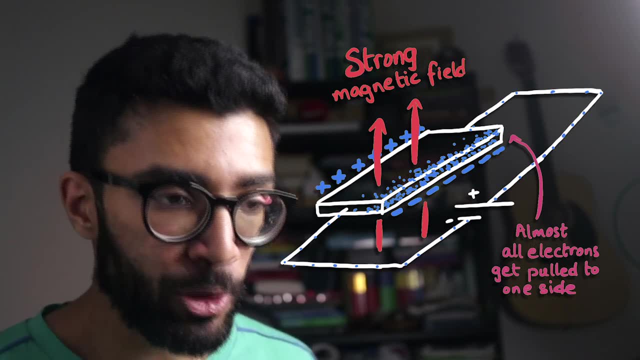 field on each one of the electrons gets stronger and stronger, And so, once again, what we're expecting is that the voltage gets larger as we increase the strength of the magnetic field. We're expecting more and more electrons to be pulled more and more strongly to the negative end. as the strength of 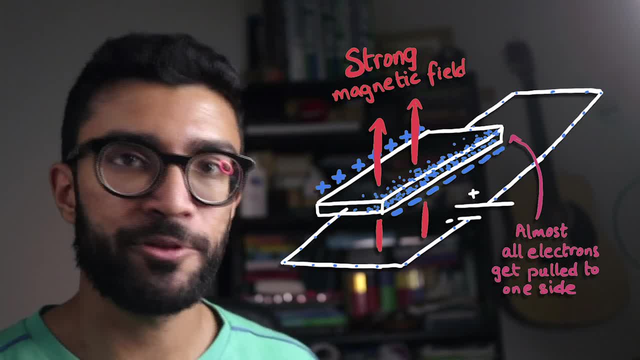 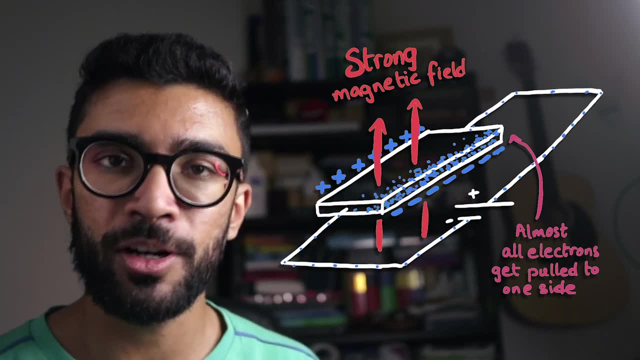 magnetic field increases, Which leaves more and more positive charges on the opposite side of the strip, And so what we have is a much, much more positive side and a much, much more negative side than before, when the strength of the magnetic field was not so high and only a few electrons were pulled to one side, leaving only a few. 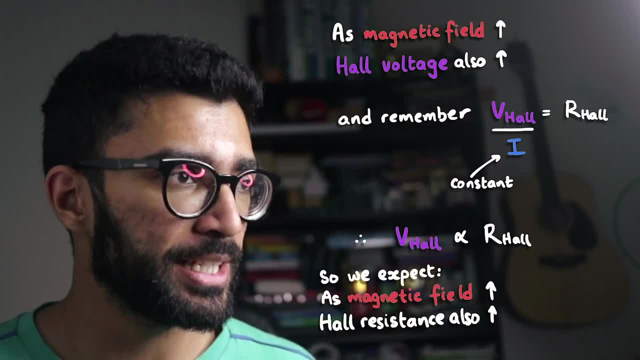 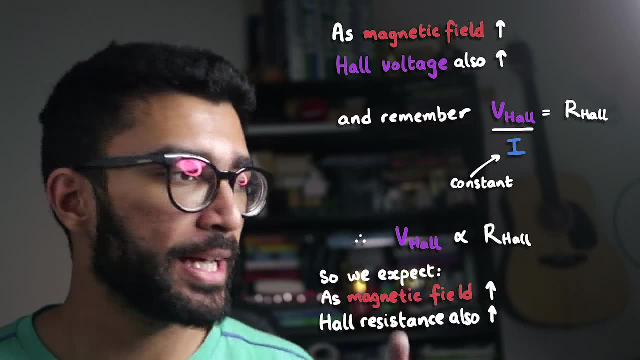 positive charges on the other side, Which means that if we're expecting the whole voltage to keep increasing as we increase the strength of the magnetic field and we're keeping the current exactly the same, then we're expecting the whole resistance to increase as well every time we increase the 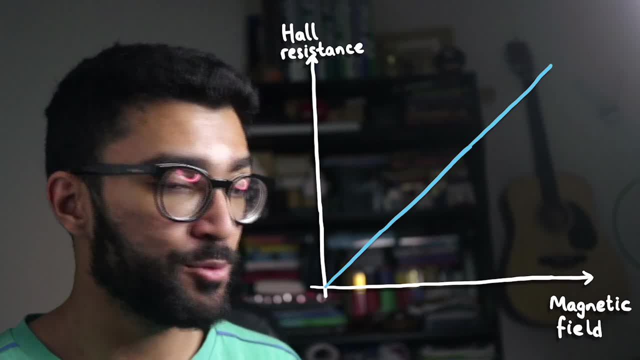 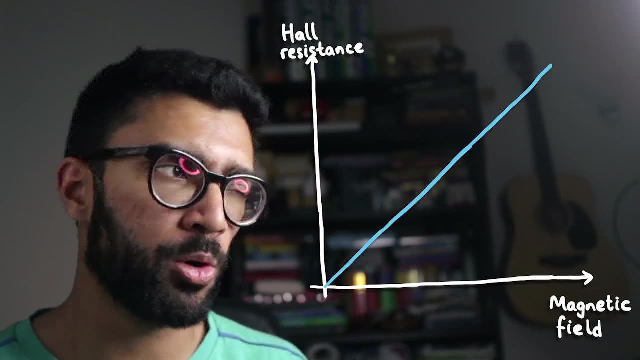 strength of the magnetic field. if we were to plot a graph, then this is what we would expect to see: on the horizontal axis, we've got the magnetic field strength, and on the vertical axis we've got the whole resistance or whole voltage. doesn't matter which you plot, because they're both proportional to each other. 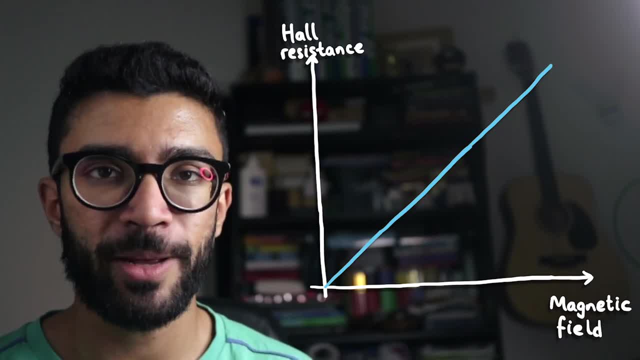 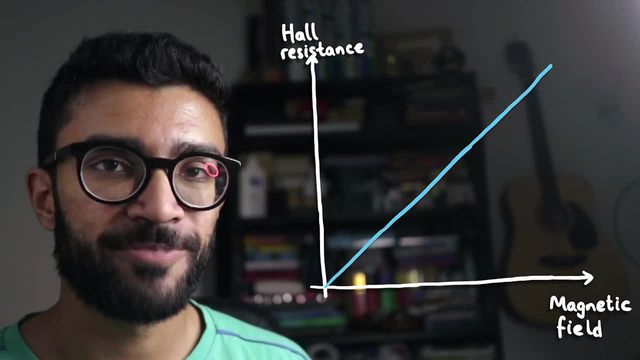 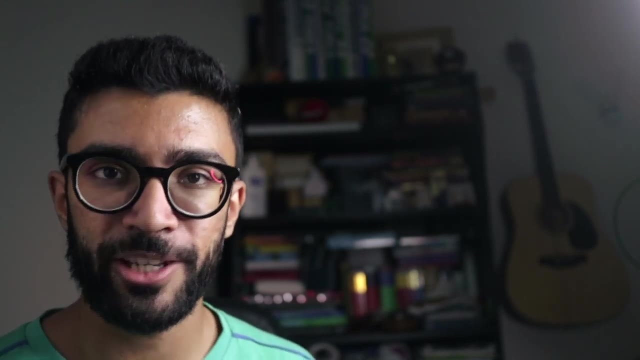 in this particular case, because we're keeping the current constant anyway. so what we're expecting is, as the magnetic field strength increases, the whole resistance increases also. and that is exactly what we see for small magnetic field strengths, because as soon as we increase the magnetic field strength, as soon as we work with strong, strong magnetic fields, this happens in. 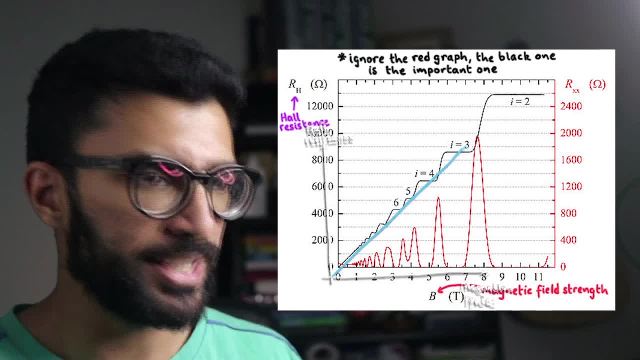 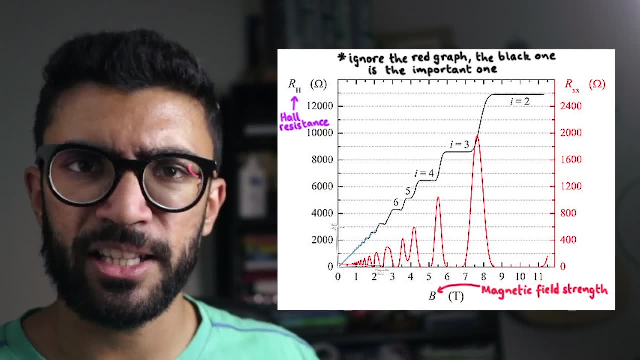 other words, the plot that i showed you earlier of what we'd expect to see is just this tiny portion of the graph and then we get flat lines in this graph and things move up, and then it gets flat again and it moves up and it gets like. this is really weird, you know, we thought it was going. 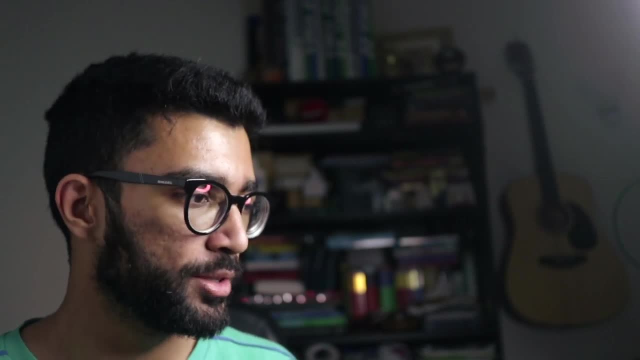 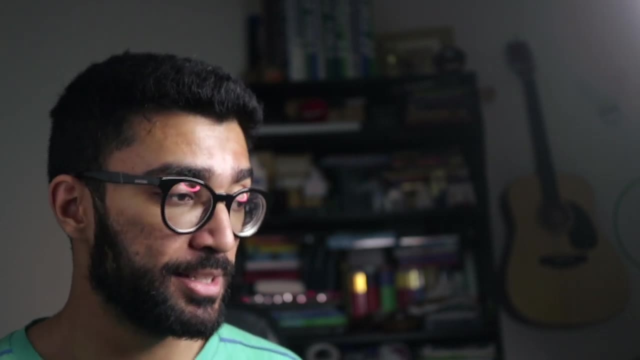 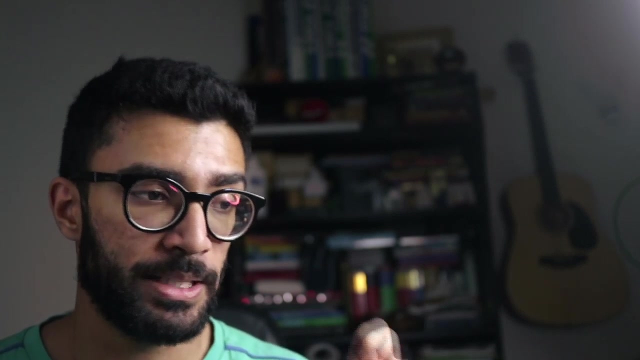 to be a simple case of increase the strength of the magnetic field. the force on the charges increases, therefore the voltage increases and so the whole resistance increases with that. we thought it was going to be that simple. we thought we're going to see a linear relationship and, to be fair, like i said, we do for small magnetic fields, but then it gets really weird. 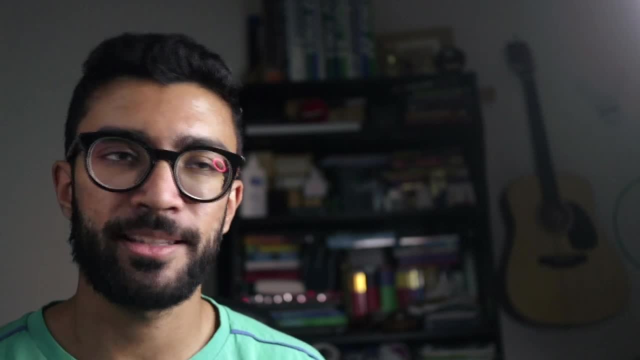 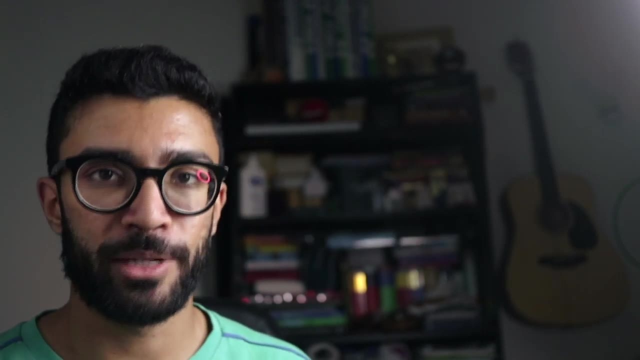 so what exactly is going on here? well, the answer to this question is, as often is the case, quantum mechanics. the logic that we use to try and figure out what we'd expect to see when we increase the magnetic field strength was based on classical physics. classical physics: 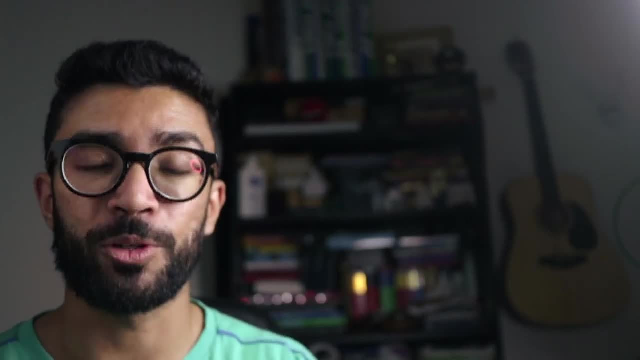 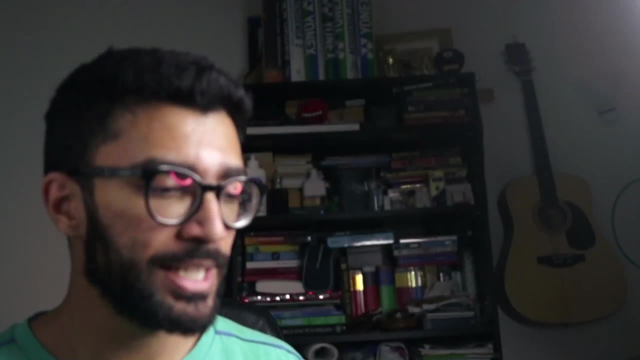 is the kind of physics that scientists used all the way up until the discovery of quantum mechanics, and it's stuff that makes a lot of sense to us. it's stuff that agrees with common sense quite a lot of the time, but unfortunately it doesn't reflect exactly how the universe 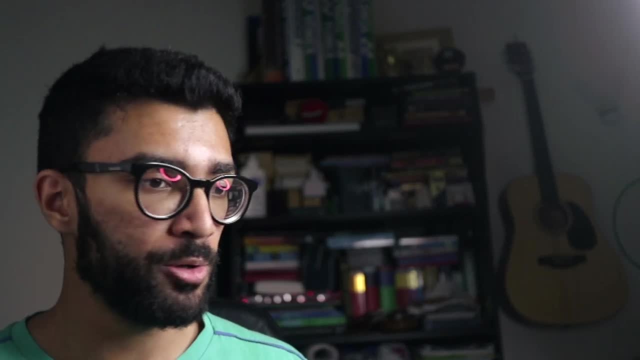 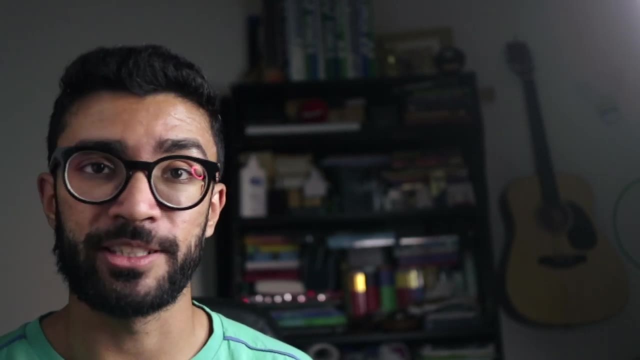 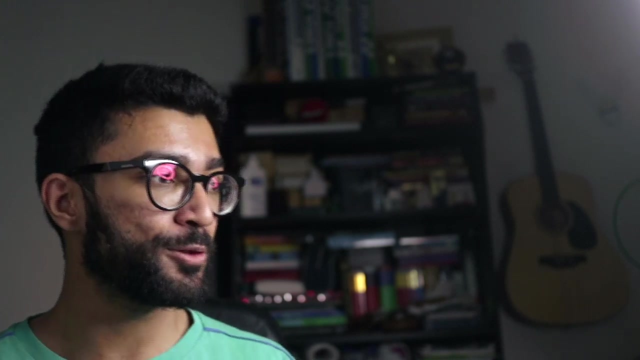 works. there are countless experiments that have been done that show the predictions of classical mechanics to be incorrect and the predictions of quantum mechanics to be correct, or in other words, experimental evidence is king. if it doesn't happen in our real universe, then it's not really that useful to us. don't get me wrong. classical physics is still useful. 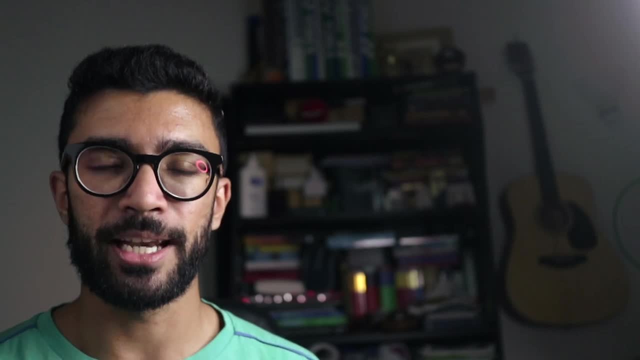 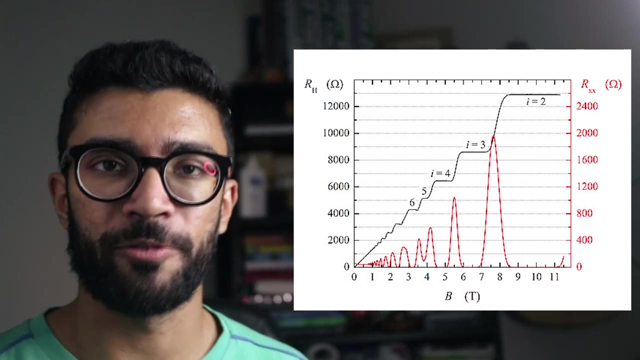 in many situations, but a much better description of the universe is quantum mechanics. anyway, that's a bit of a tangent. let's go back to what we were talking about now. what actually happens in order to give us this graph, what actually happens in our strip of metal is: 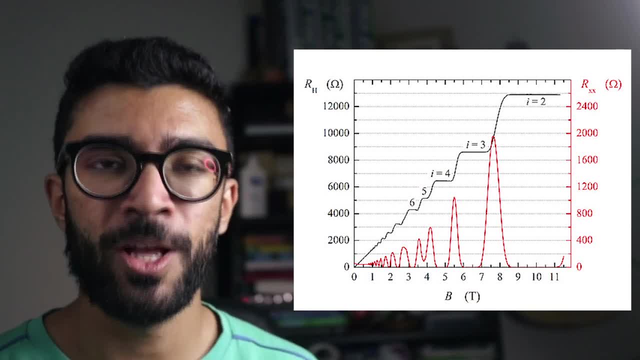 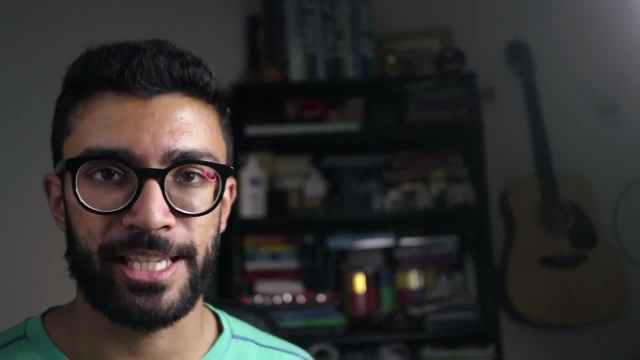 quite complicated, and the quantum physics behind it is quite complicated as well. so i'll try and describe it to you by using an analogy, and i'll try and show you the kind of thinking we need to have in order to understand what actually happens. now this analogy is: 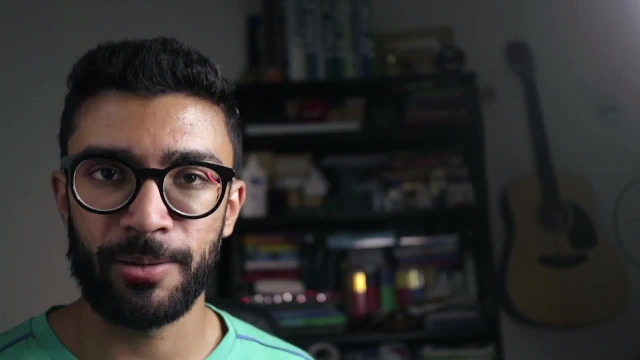 going to be based on atoms and, more specifically, the internal structure of atoms. many of you may have seen in high school physics and chemistry that atoms are made up of protons, neutrons and electrons. we've already discussed that in a previous video. we've talked about the 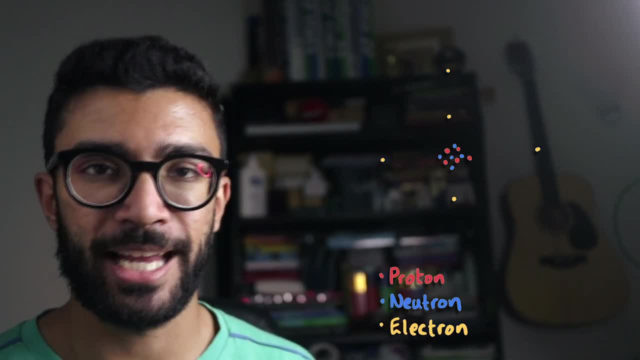 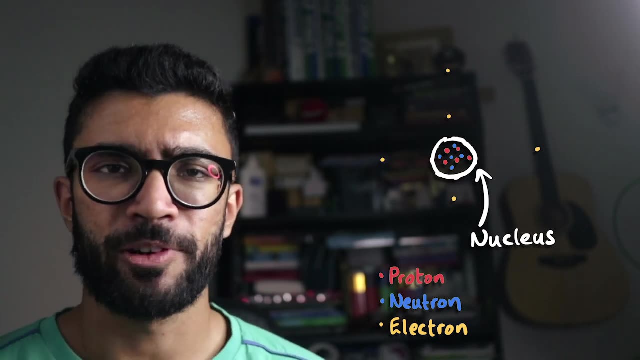 structure of electrons and neutrons, and we've already discussed the electrons when we were discussing our metallic strip. but in addition to this, protons and neutrons are located at the center of the atom, in a region known as the nucleus. but that's not relevant to us right now. what we care about is the structure of electrons around the nucleus. 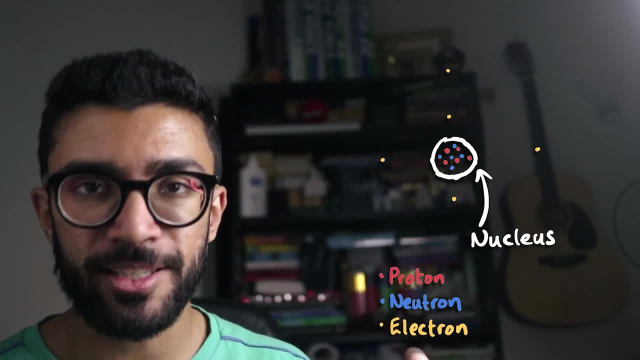 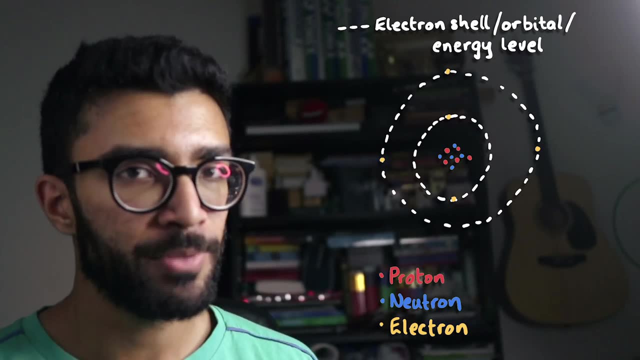 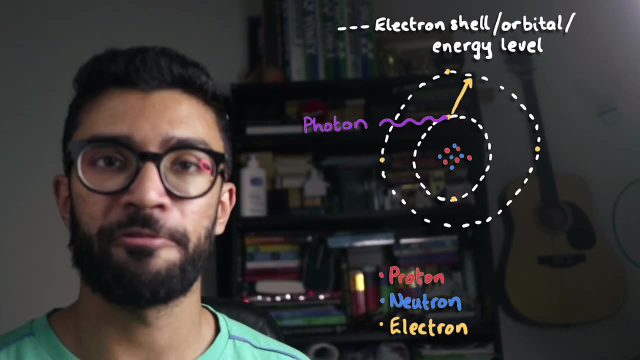 now, many of you might know that electrons can only exist very specific distances away from the nucleus. these are known as electron shells or orbitals. however, interestingly, electrons can move from one shell to another by means of either absorbing or emitting what's known as a photon, a little particle of light anyway, so electrons. 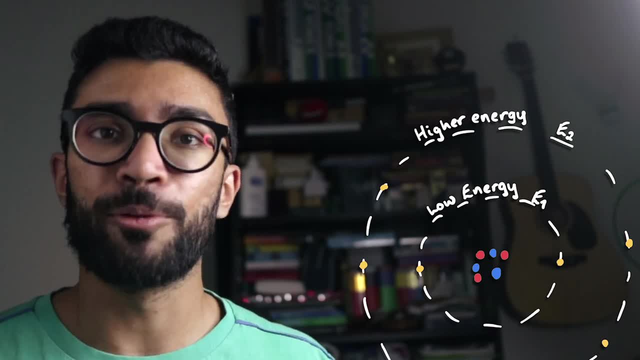 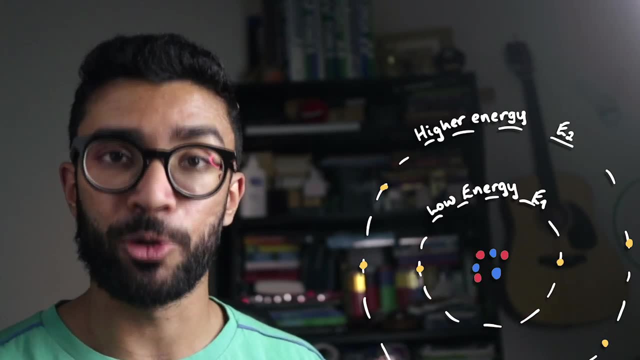 can move from one shell to another, and if they're moving to a shell that's further away from the nucleus, then the energy of the electron increases, because shells closer to the nucleus are lower in energy, they're more stable, and so moving to a shell that's further away from 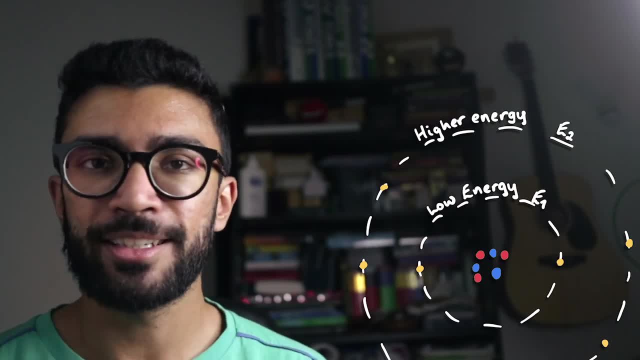 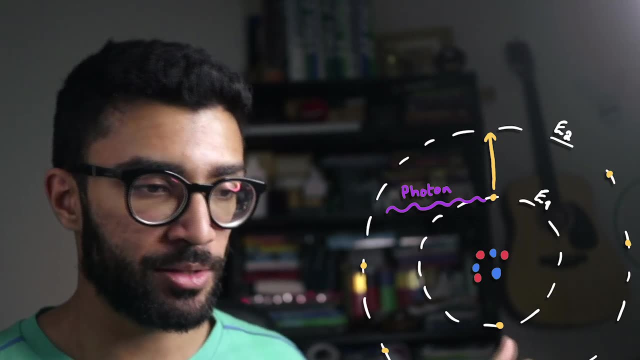 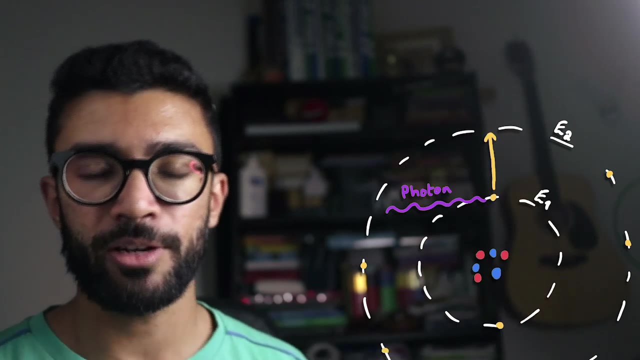 the nucleus means an increase in energy of the electron. where does this energy come from? well, the electron absorbs a photon of light. that photon itself is energy, because lightwaves are just propagating energy. and then, when this photon is absorbed, the electron can move up to the shell above or another shell that's further up. however, the important thing is: 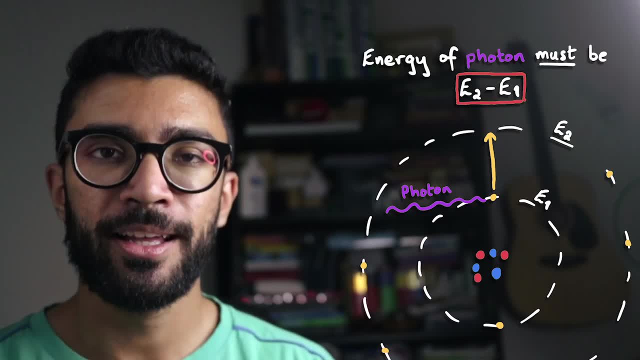 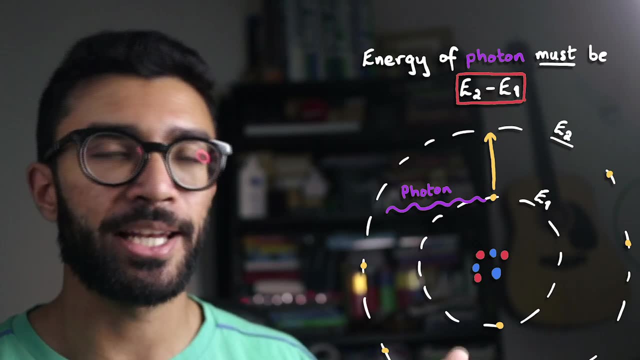 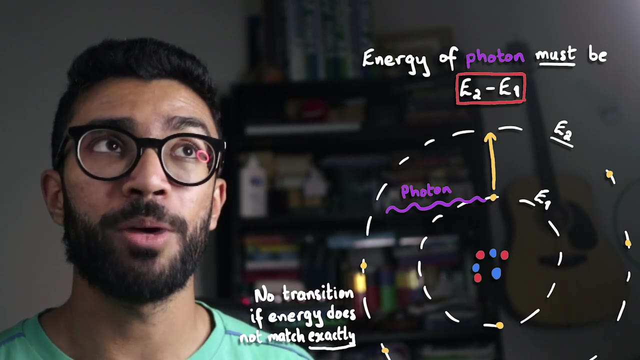 that the photon must be of a very, very specific energy. this energy of the photon corresponds to the difference in energies between the energy of the electron in the lower shell and the energy of the electron in the upper shell. in other words, the electron needs to get that very specific amount of energy in order to get up to the next shell. too much 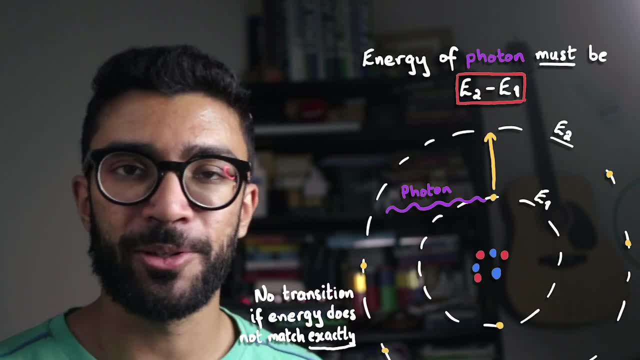 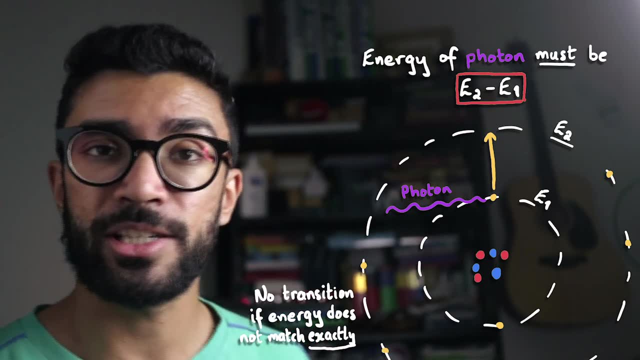 and too little, and the electron will not transition. the photon will not transition, the electron's will continue on its way, not interacting with the electron, and the electron will stay exactly where it was. so we can imagine an experiment where we've got photons, initially of a very 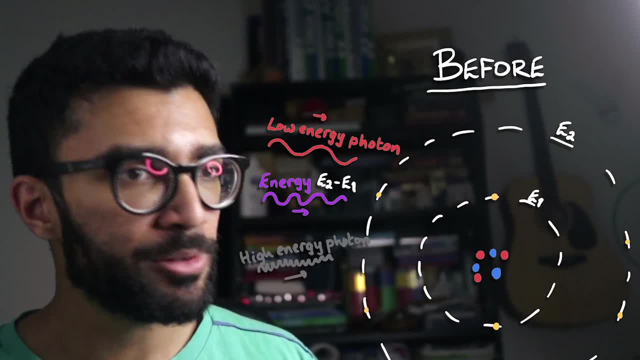 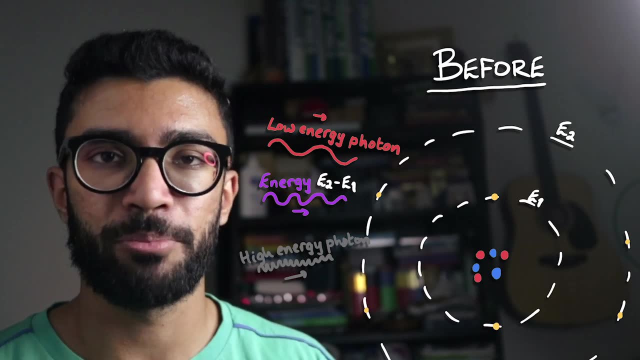 low energy being fired towards our electron and then we increase their energy and see what happens. what we're going to see is that very low energy photons come in and, you know, nothing happens. the electron doesn't jump up to the energy level because the energy of these photons is not quite. 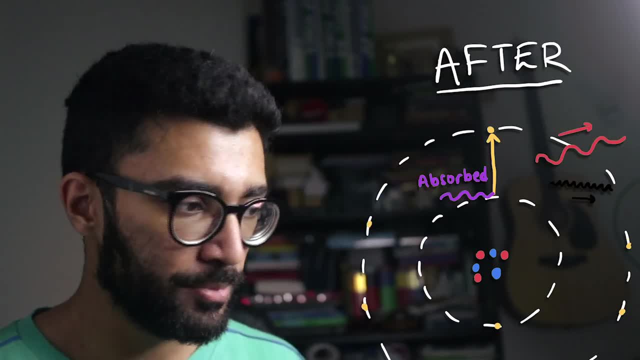 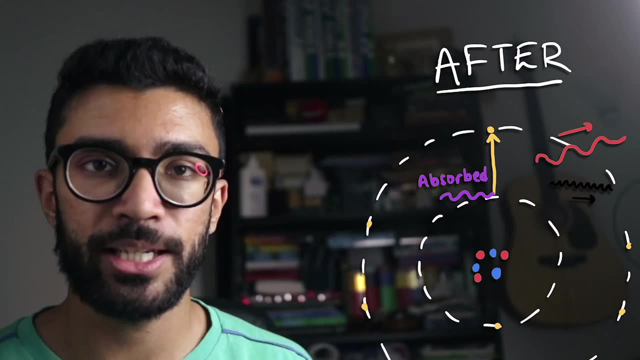 right and then at a very specific energy the electron does jump up to the higher energy level and then if we bring in electrons back to the lower energy level and we keep increasing the energy, then even photons with too high energy do not cause the electron to jump up to the next shell because, like i said, 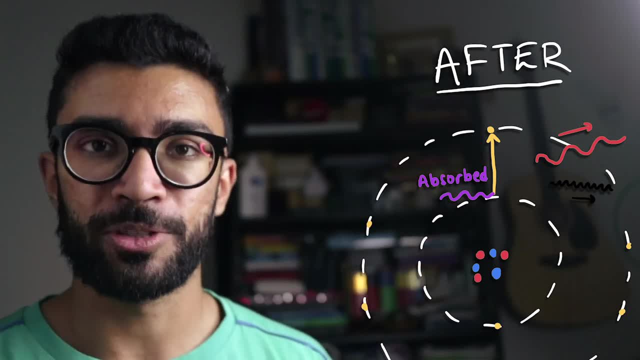 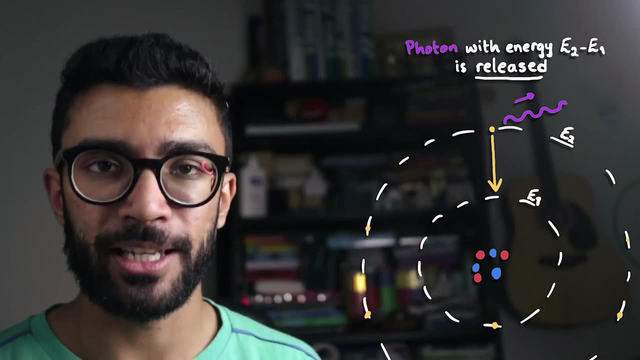 the energy needs to be exactly right. keep this in mind. this is really important for in a minute, but just as a quick finisher to what we've just been discussing, electrons can also move down from a high energy level to a lower energy level, or higher shell to a lower shell, by. 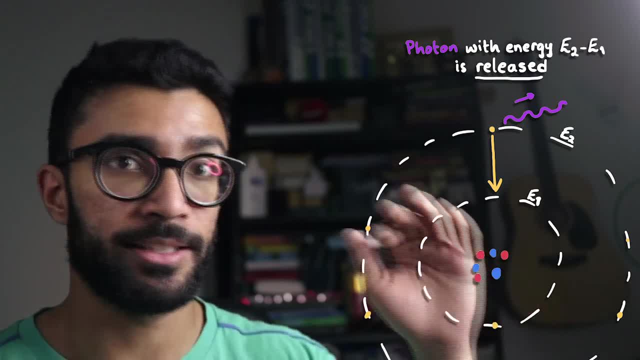 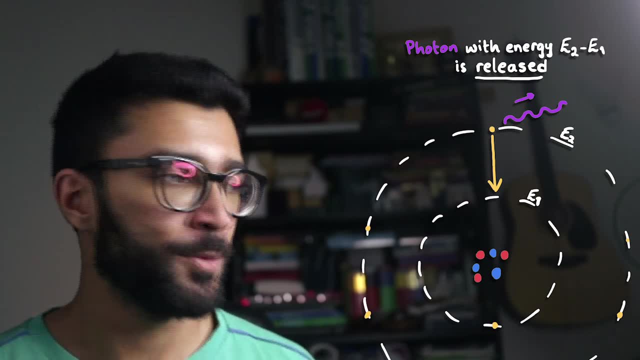 releasing a photon of that very specific energy: the energy. that's the difference between the energy of an electron here in the higher shell and the energy of the electron here in the lower shell, anyway. so, coming back to the important thing, we saw that as we increased the 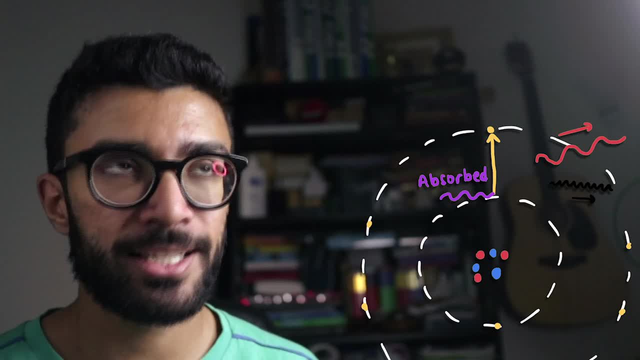 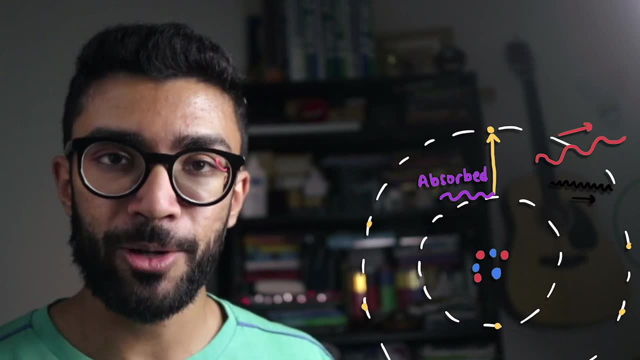 energy of the photon. nothing happened until the energy was just right. and then, when the energy was just right, the electron transitioned from the lower shell to the higher shell, and then coming back to an electron in the lower shell. we kept increasing the energy, so that the energy was. 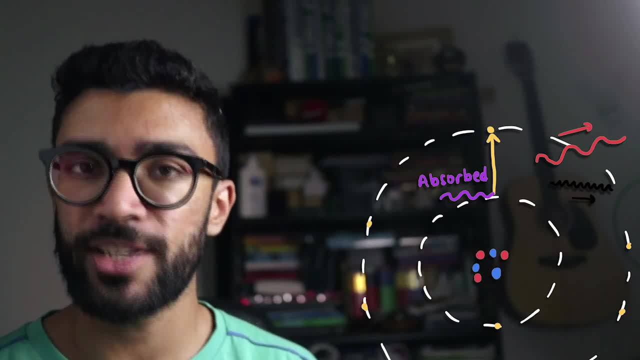 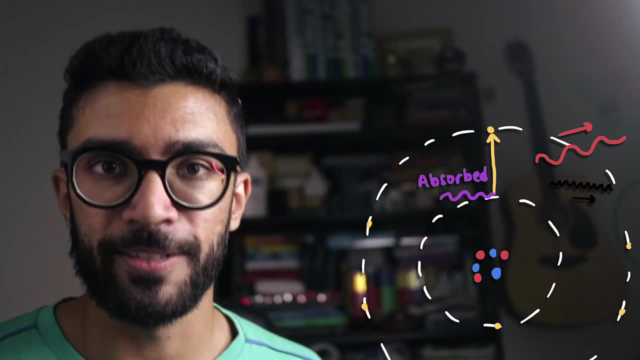 larger than the difference between the energies of the two shells, and still nothing happened. in reality, things are a little bit more complicated, but we won't go into that here. the idea is: what's important because it's this kind of thinking. that's what's important because it's this kind of thinking. 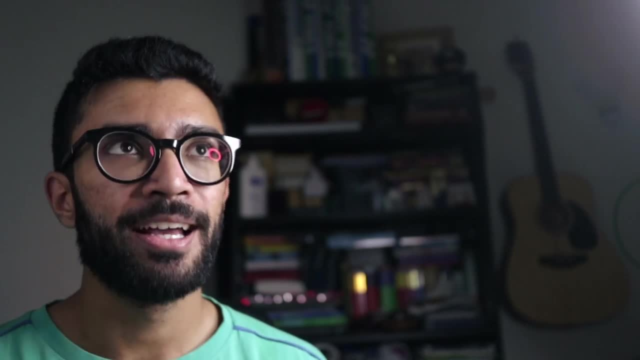 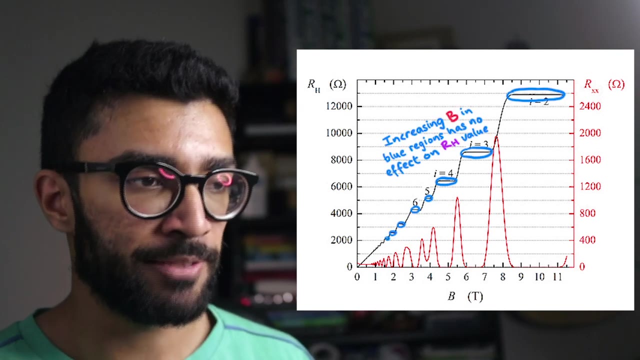 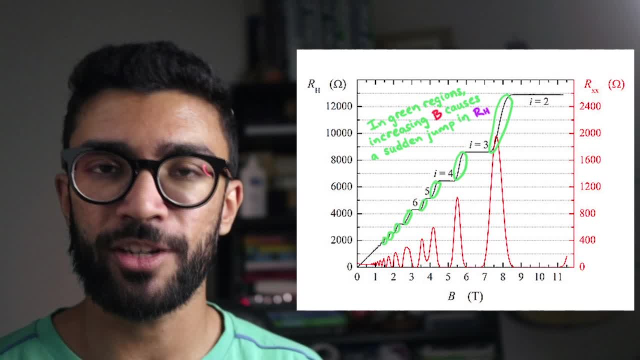 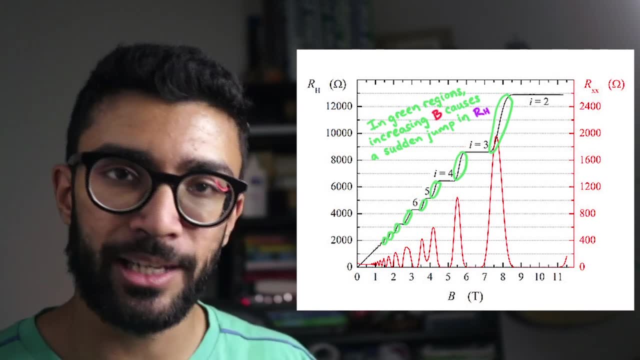 same, and then it jumps up to the next value of the resistance. just like the electrons jumping between energy levels, we needed the photons to be of the exact right energy, and increasing this energy a little bit didn't make any difference. we just needed those specific values. this is exactly what. 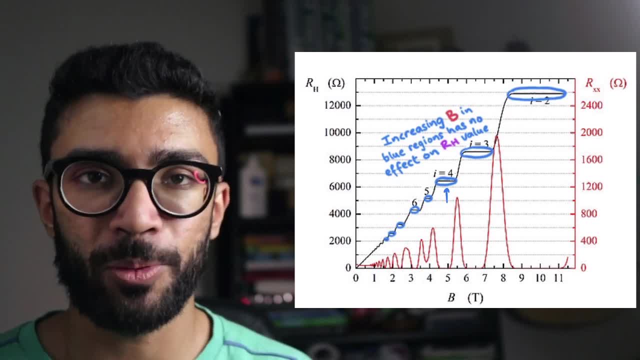 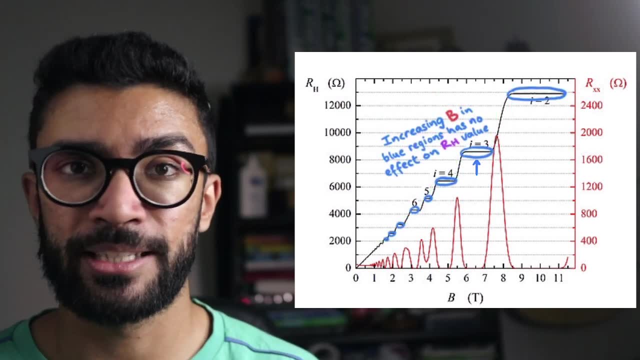 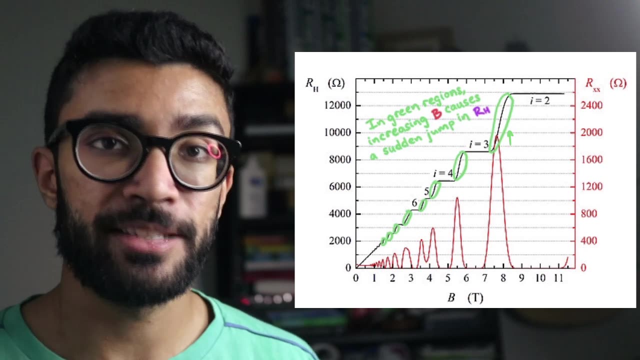 we wanted to stop earlier, but, kID, this is just another way to have our experiments get started. so the first thing we're going to do is we'll start with the magnetic Popular strip that we'll use as our bridge against the detector, and it's not going to be vivid. 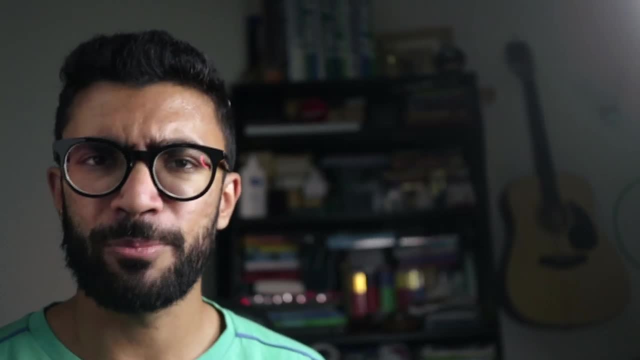 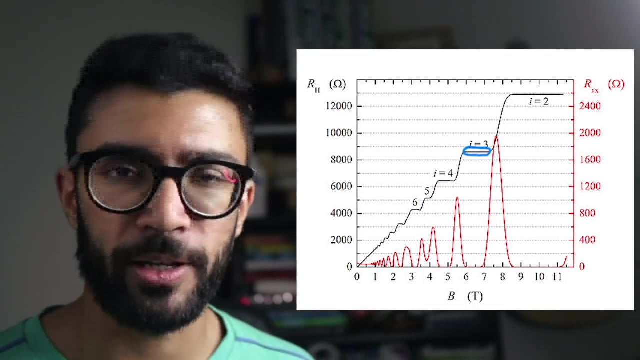 even with trees, only so what we're going to do. we're going to explain what's happening in the skeleton, but first of all we're going to observe fields and then we're going to start with cool, and this is that straight line, or this one, or this one, or this one, because along those flat lines, 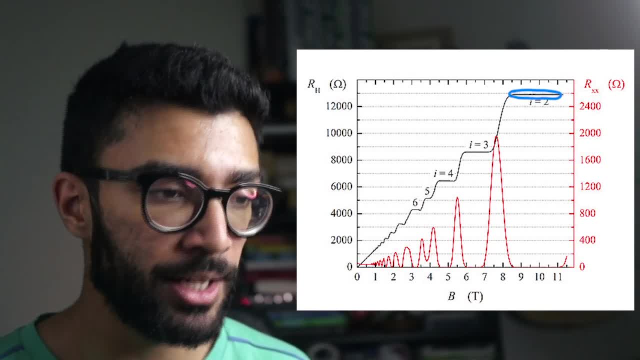 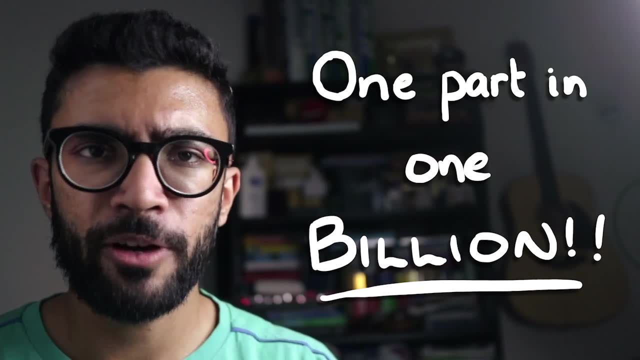 the values of the Hall resistance are identical to each other for different magnetic fields, to within one part in a billion, like they are as close as they can get, and I don't know if I've stressed upon you just how mind-blowingly amazing that is. so let me even clarify to you that these 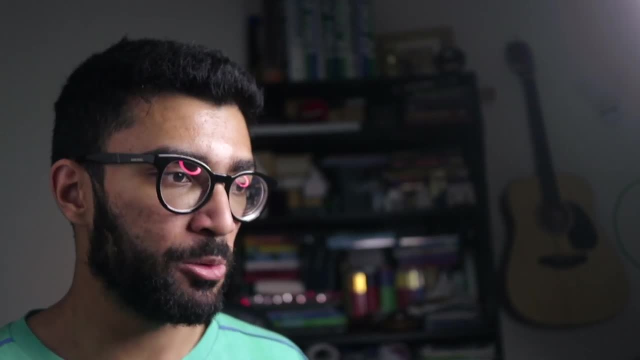 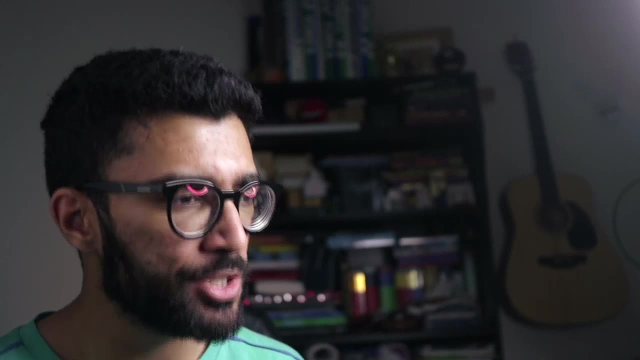 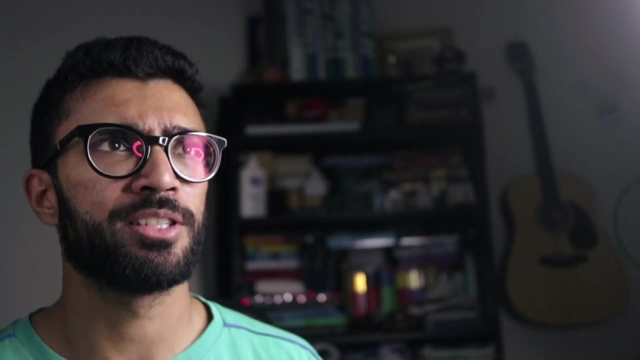 values, these amazingly close values, were got with a sample that was dirty and sort of not broken but just sort of damaged and sort of ugly looking. it wasn't a perfectly polished, you know, perfectly flat surface that was supposed to be in very specific conditions. the experiment was almost. 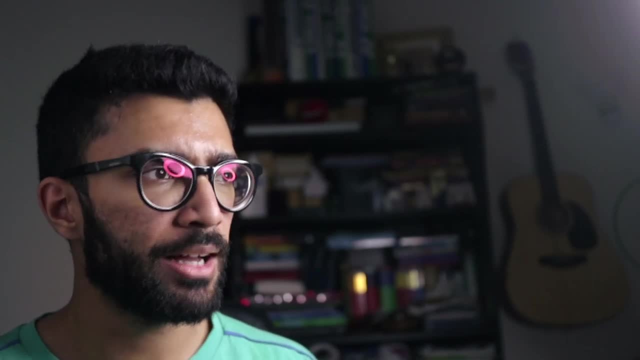 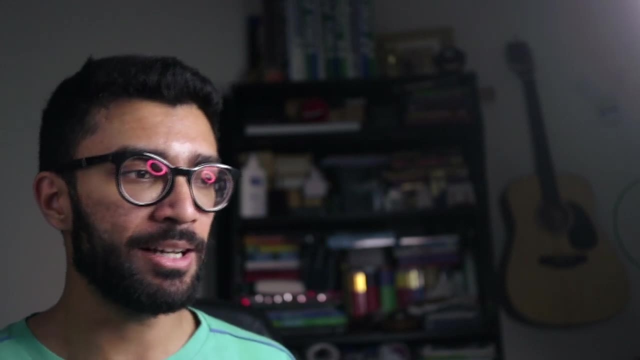 done in a very throwaway way. the idea is that often when you do experiments, things are very, very messy. the real world, the real universe, is extremely messy compared to what we see in the beautiful maths that's written down here and that's what we see in the real world. 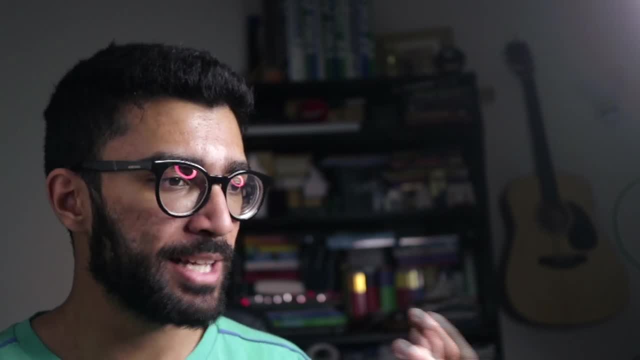 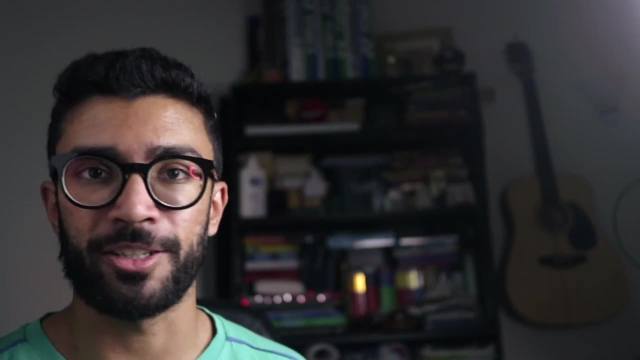 in all our theories we expect things to go a very specific way, but when we take readings and results, there's a lot of errors that go into measurement: errors, human errors, random errors, systematic errors that we haven't considered, so on and so forth that result in our experimental 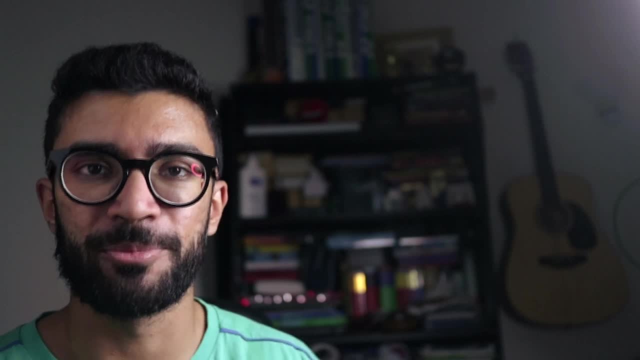 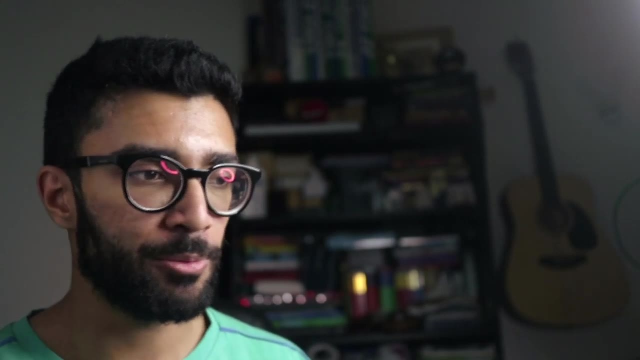 readings being sort of not so clean, not as clean as we expect them to be anyway, and so that's why this particular set of results is so amazing. regardless of how nicely we've set up our experiment and how cleanly we've polished our sample, our little metallic strip, we're getting 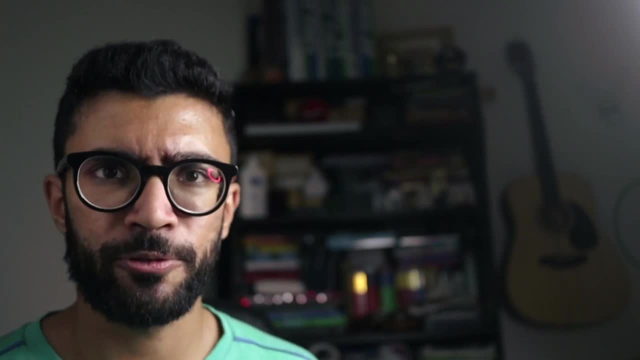 these values accurately and we're getting these values accurately and we're getting these values accurate to within one part in one billion. if we draw a line straight through them, that is about as straight a line as we can get. and another interesting thing is that the value of the 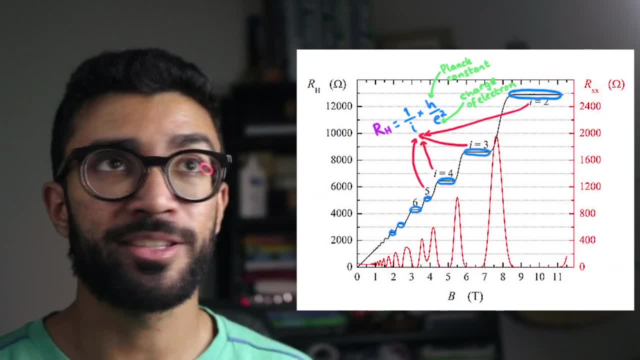 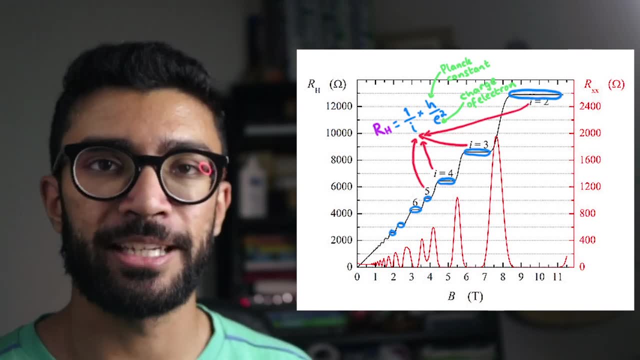 whole resistance at all of these plateaus is equal to some simple fraction multiplied by constants of nature: the Planck constant, which is a fundamental constant in quantum mechanics, and the charge on an electron. and this is quite cool as well, it's not just some random numbers. 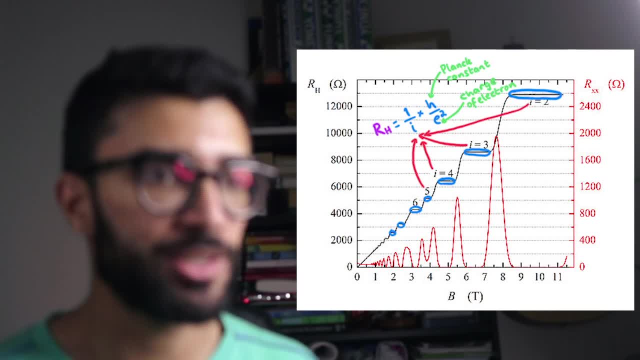 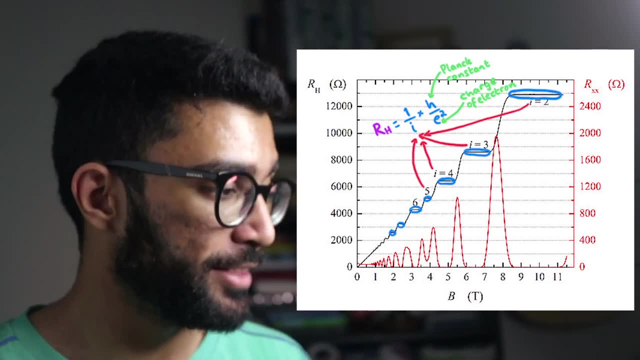 some random resistances. they are very specific fractions multiplied by some very specific constants of nature, and that's quite a cool thing as well, but anyway, so that's just an aside. the main thing is that these lines are so, so straight, and therefore, for that reason, these 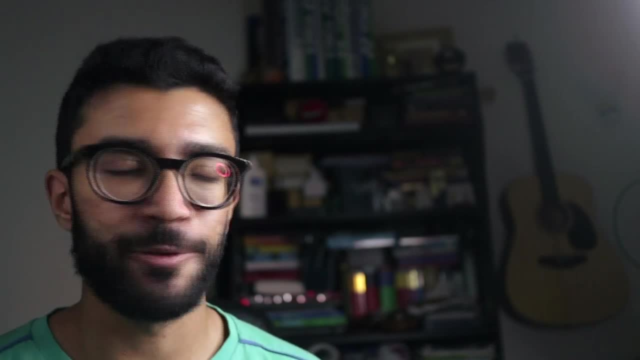 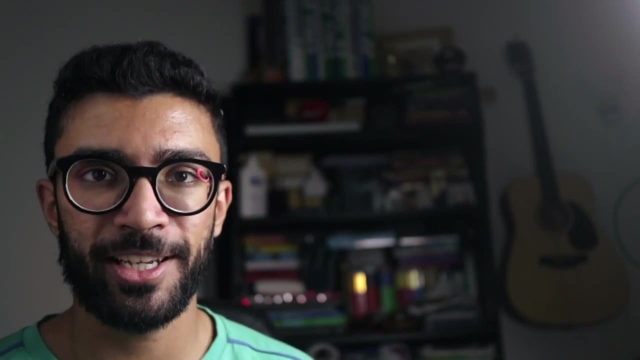 lines are my nomination for the straightest lines ever measured. like i said, if you've got any better examples, then chuck them down in the comments below. i really definitely want to read about them, because this is the kind of stuff that i enjoy and if you want to know a bit more about. 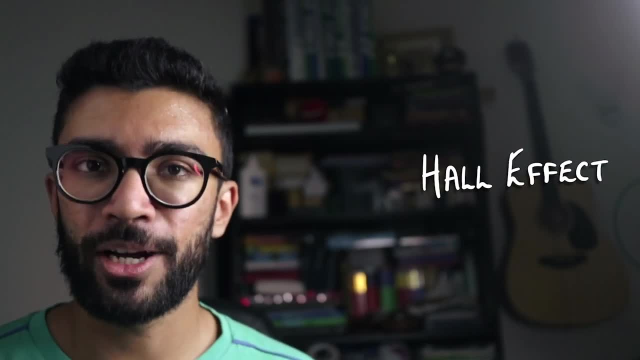 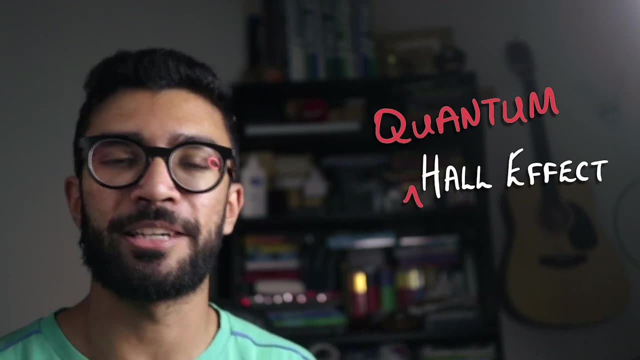 the hall effect. check out the whole effect on wikipedia. if you're feeling brave, check out the quantum hall effect, which is even more complicated. and if you really want to blow your mind or just read a wikipedia page and not understand a word it says, then check out what's known as the integer quantum hall effect and the fractional quantum hall effect. 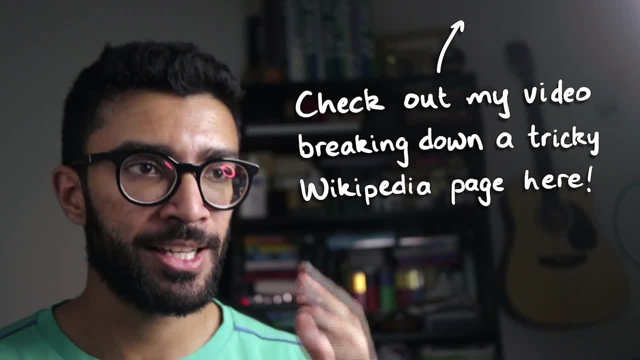 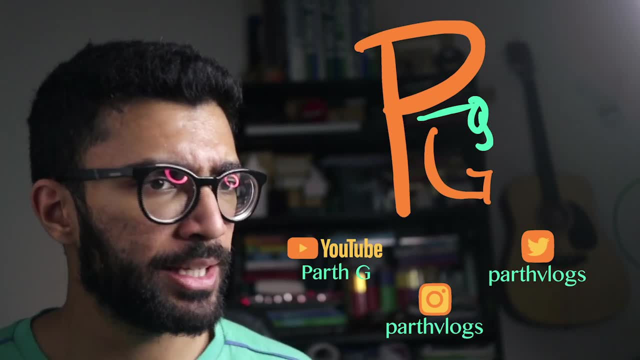 and lastly, i just want to quickly mention that i love making videos like this because a lot of these topics are stuff that i struggled with when i was at university. my Maxwell's equations videos were made because i remember thinking while i was at university, these equations, 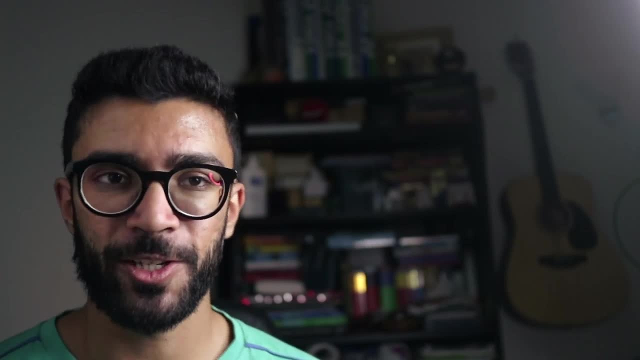 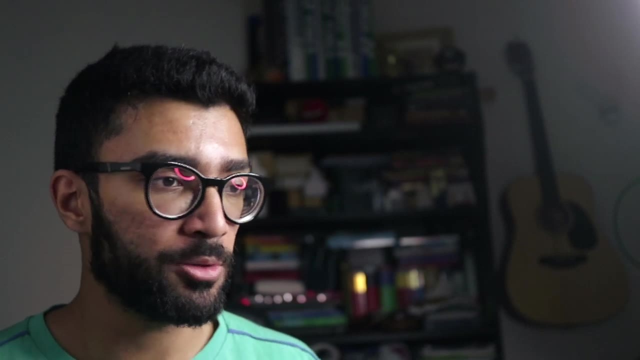 are quite challenging. i haven't fully got the grasp of them and having made those videos, i know that i haven't got the grasp of them. but i understand more about them, and the same is true about quantum hall effects and why i love them so much. so i'm going to go through them one by one. 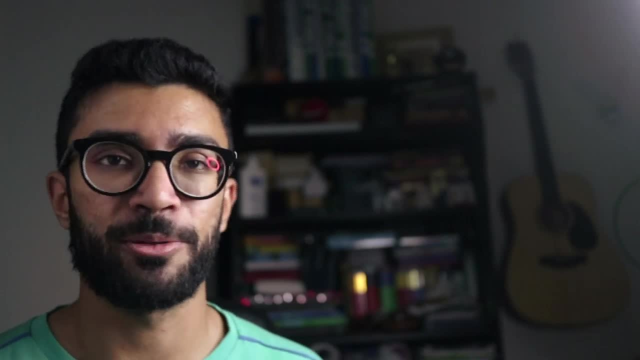 and i'm going to start with the quantum hall effect, which is something that i never had time to get my head around while i was studying at uni. it was just something that was mentioned briefly and we moved on, and there were exam questions about it and i would avoid them every.